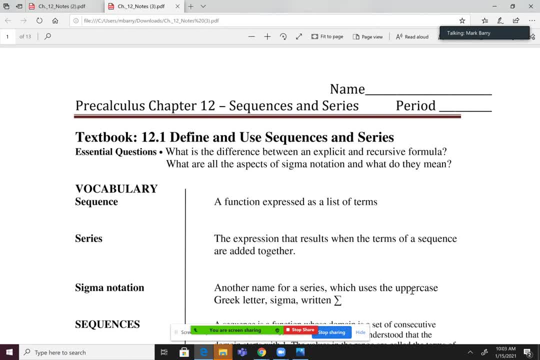 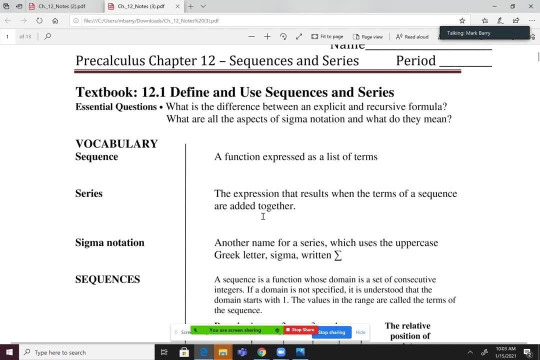 okay, And they're kind of fun, as fun as math can get right, So let's go through it, okay? So what is a sequence? Well, a sequence is a function expressed as a list of terms. okay, So it's a list of numbers. Let me make a sequence for you right now: 3, 6,, 9,, 12,, 15,, 18,, 21.. 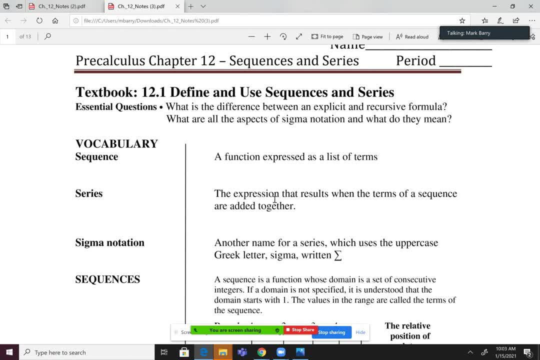 That was a sequence. Did the sequence have a pattern? Yes, yeah, and most sequences do have patterns, although even if it didn't have a pattern, it would still be a sequence. okay, There's actually a very famous sequence that has no pattern: the digits of pi. If you read those up, 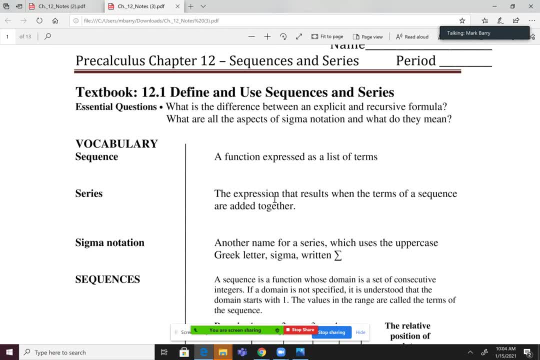 3, 1,, 4, 1, 5, 9,, 2, 6,, 5,, 3, 5, 8, 9, 7, 9, 3, 2, 3, 8, dot, dot, dot. That's actually a sequence with no pattern, but it's still a sequence, if you. 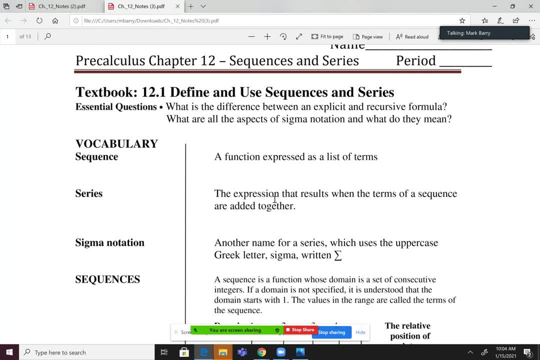 list them out like that. For those of you wondering how I know those digits of pi, I actually don't have pi memorized very well. I have like six digits of pi memorized but I have a poster of all the digits of- or not all of them, but I have a poster of about 30 digits of pi in my room. 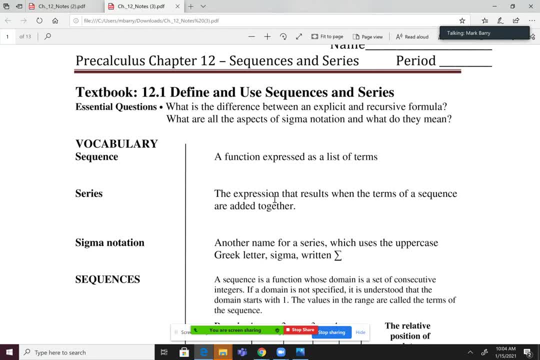 so I was actually just reading that off there. okay, Okay, so that's what a sequence is a list of numbers. okay, A series is the expression that results when a- the terms of a sequence, are added together. So we're going to see there's times where it's 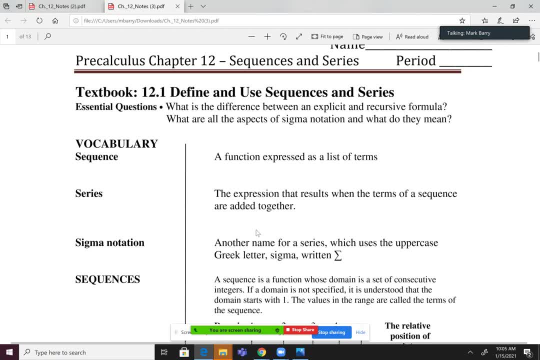 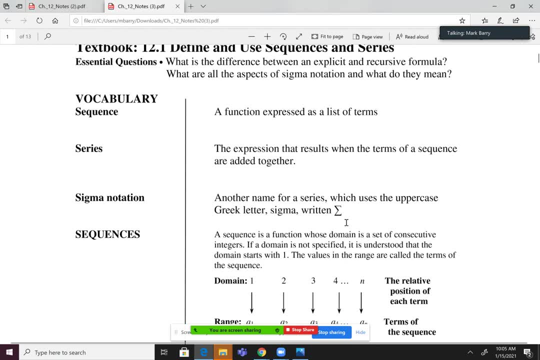 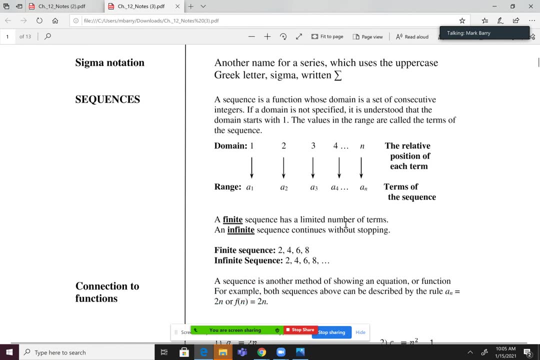 beneficial to add all these terms together and we call that a series. We also call that a sigma. It's the Greek letter, right here It looks like a funky E. That means the same thing as series. It means add all these terms up. okay, All right, cool. So let's talk about sequences more. 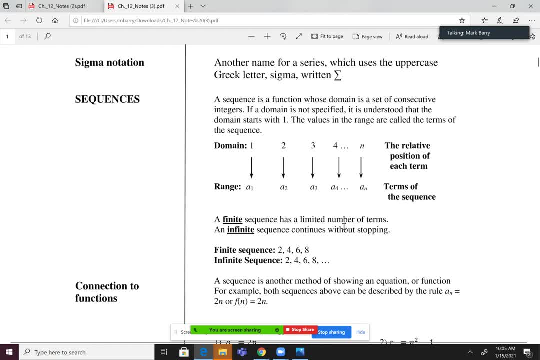 So, like we said, a sequence is kind of like a function, but the key difference between these, the key kind of distinction on these functions, is that the domain is a set of consecutive integers. okay, So domain is what we plug in, correct? 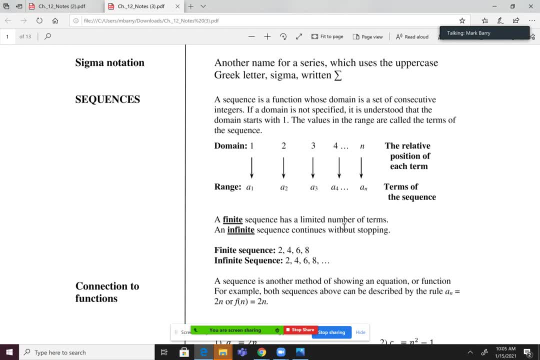 So when we had regular functions, were we allowed to do like f of 0.5 or f of 3 over 2? Yeah, we were correct. But on these functions, sequences, we're only allowed to plug in integers. okay, And we are usually starting by plugging in one. That's the first integer we 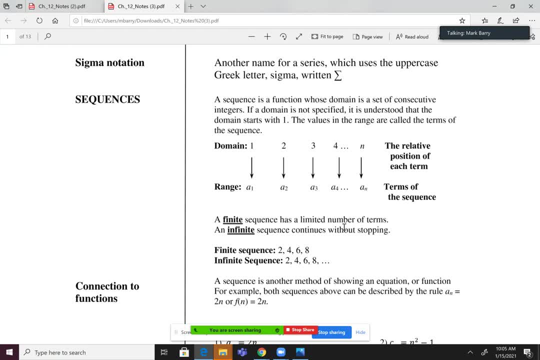 plug in and then go up from there. okay, Consecutive integers. Now it is possible to start with other numbers, like 0 or maybe 2, but for the most part- generally speaking, about 90% of the time- you're going to start by plugging in a 1,. okay. 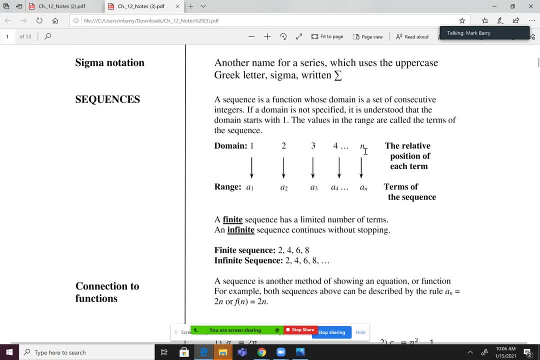 So the domain would look like this: 1,, 2,, 3,, 4, and n, And n is going to be like our main variable here for domain. okay, Now for normal functions. x is the main domain variable, right, X is usually. 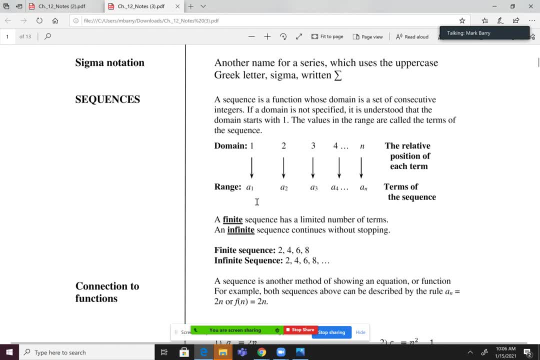 what you're plugging in. In this case, we call it n, The range. the output, okay, looks like this: A and then a subscript 1.. I'm going to be reading that, and most people read this as a sub 1,. 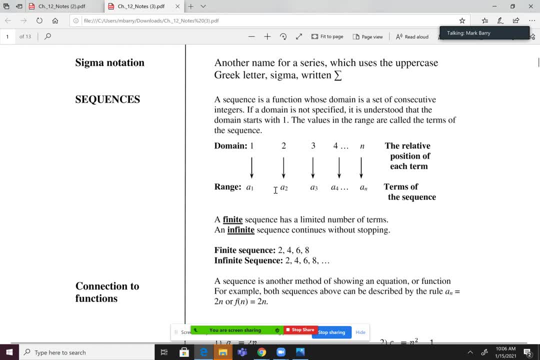 okay, Because it's a subscript of 1.. A sub 2 would be the second term in the list, A sub 3 is the third term, A sub 4 is the fourth term And a sub n is the nth term. Got it Okay, We'll also be. 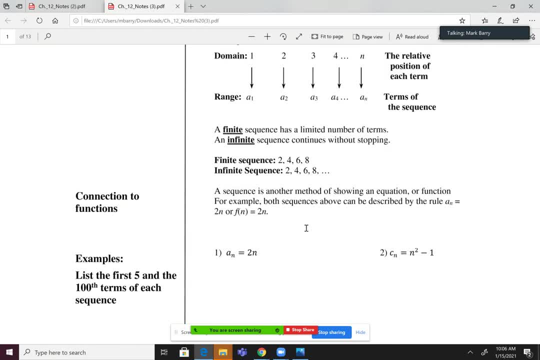 looking at two different types of sequences: infinite sequences which go on forever. and then the opposite of that, which is the infinite sequences which go on forever, That word up there which I would guess if most of you said it out loud right now. 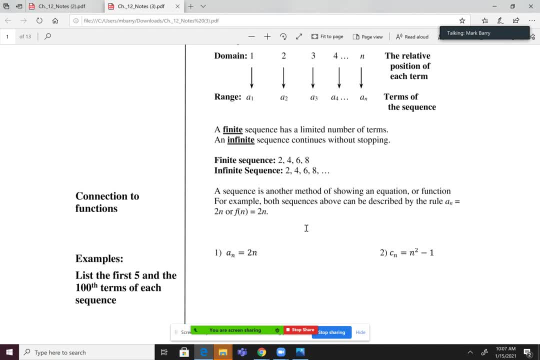 you'd pronounce it wrong. That is finite sequence. Yeah, most people think that's pronounced finite, which makes sense, because if it's infinite, then it should be finite, right. But it's not. It's finite. So finite means it ends, right. There's an ending point to that sequence, okay, Awesome. 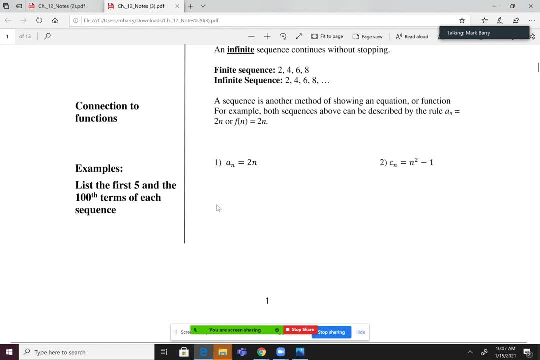 So let's take a look at our first two examples here of sequences And our goal to start off easy here for the first couple problems. okay, Is it going to get a lot harder after that, You bet, But it's going to start off nice and easy, okay. So what they want here is the first five terms. 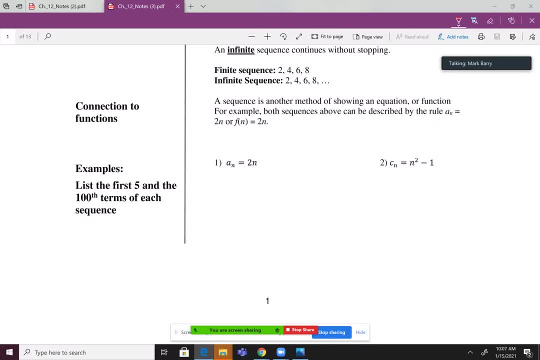 and then the 100th term. So to find the first term, the first term is called a sub 1.. And a sub 1 equals and just like functions. if the subscript over there is a 1 for n, that means I plug in a 1 for n on the right side. So a sub 1 is 2 times 1, which is 2.. 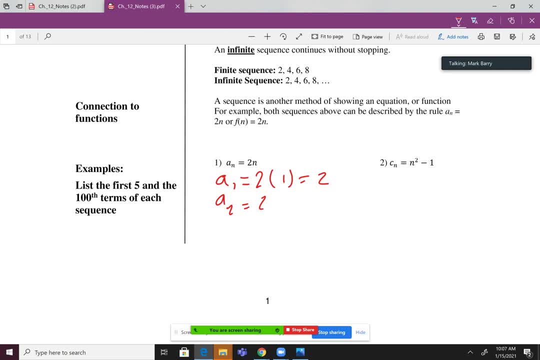 A sub 2 is 2 times 2,, which is 4.. A sub 3 is 2 times 3,, which is 6.. A sub 4 is 2 times 4,, which is 8.. A sub 5 is 2 times 5,, which is 10.. 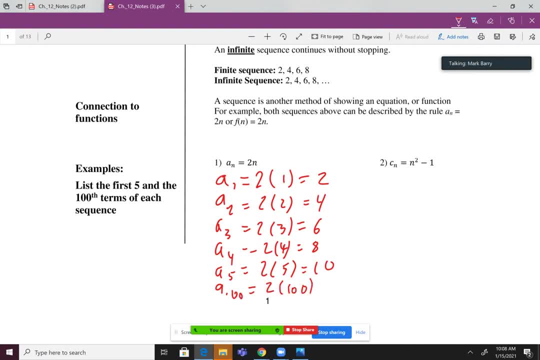 And a sub 100 is 2 times 5,, which is 10.. And a sub 100 is 2 times 5,, which is 10.. And a sub 100 is 2 times 100,, which is 200.. 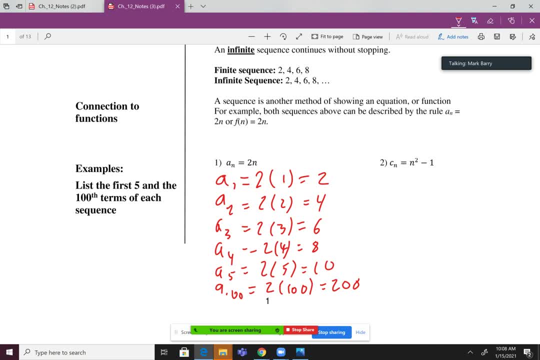 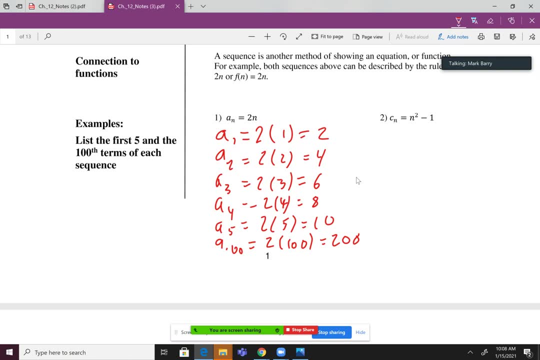 The first five terms and then the 100th term. okay, If we're technically going to write this as a sequence, which I would like to do, you would, like I said earlier, write it as a list of numbers. So I'll go ahead and do that. So I'd say 2, 4,, 6, 8, 10,, dot, dot, dot, 200. 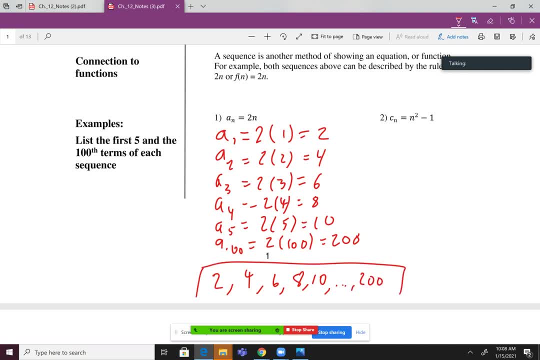 200.. The first term, a sub 1 is 2.. The second term a sub 2 is 4, and so on and so forth. Not too difficult, right? Okay, let's go ahead and try number 2.. Shouldn't be difficult either. 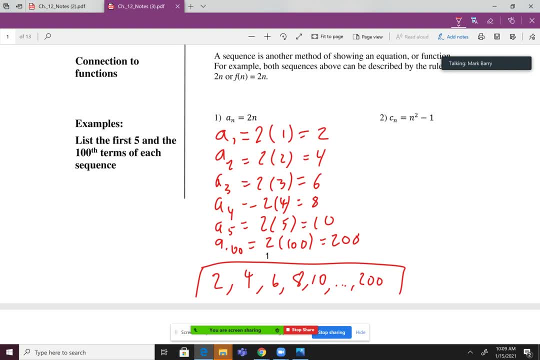 You can see that they call this one c sub n. So, just like you know, for functions usually we use f of x, but you could also use g of x or h of x, Like you can just call it a different letter, right, But the idea is the same. So c sub 1,. 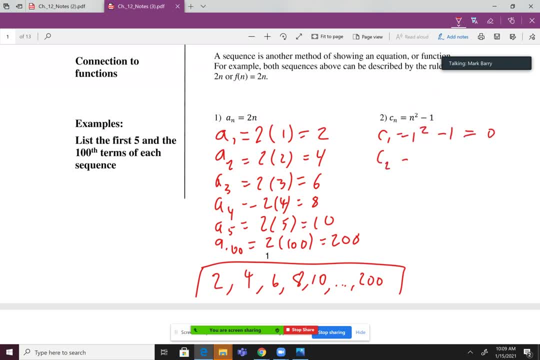 1 squared minus 1.. So that's 0.. So c sub 2 would be 3.. C sub 3 would be 8.. C sub 4 would be 15.. C sub 5 would be 24.. C sub 100.. 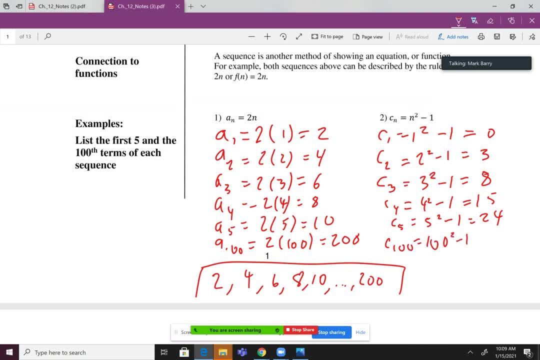 100.. 100 squared is 10,000. So this would be 9,999.. So my list here would be 0, 3, 8,, 15,, 24,, dot, dot, dot, 9, 9,, 9,, 9.. 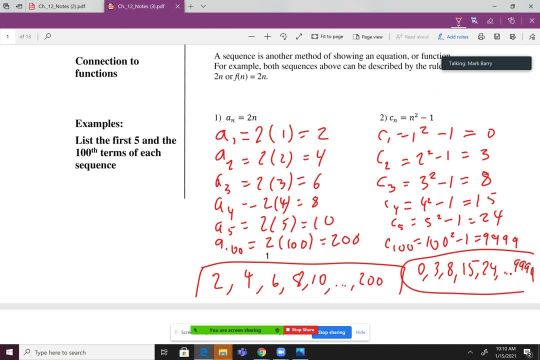 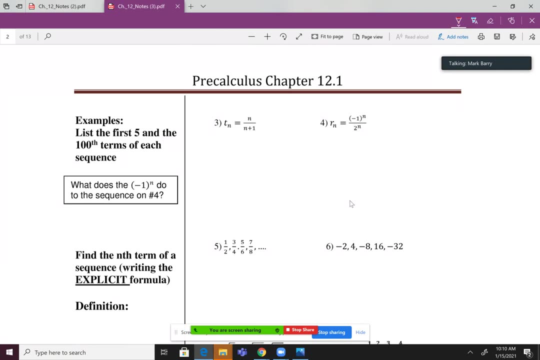 Beautiful, Great list of numbers. we got going there right. All right, let's go to the next page, where I think it's still going to be pretty easy here, Same idea We get: t sub 1 is 1 over 1 plus 1.. So that's 1 over 2.. 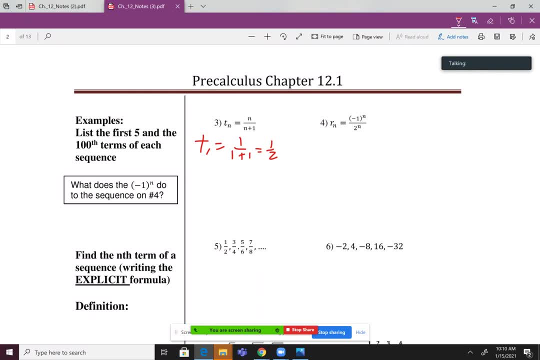 So that's 1 over 2.. t sub 2.. 2 over 2 plus 1.. So that's 2 over 3.. I'm actually going to stop right there, because I know what's going on here, right? I don't need. 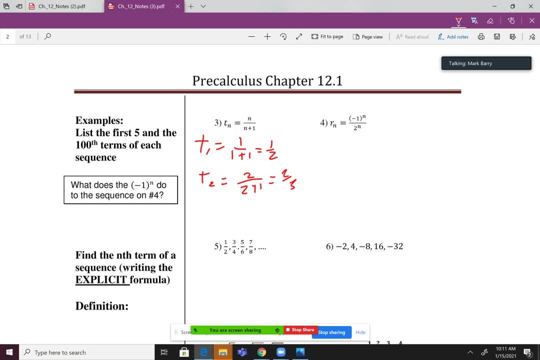 to show my work anymore, because I can make this list in my head. now You guys see what I'm saying. Every time the top number is whatever number we're on, So that's 1.. And then the bottom number, the denominator, is 1 more than that, So then I have 2 over 3.. Then it's going to be 3,. 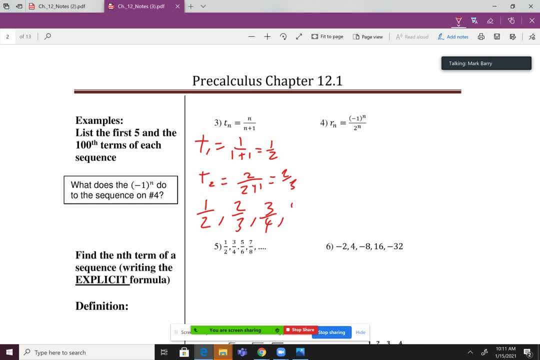 3 over 1 more than 3.. So 3 over 4, 4 over 5.. The top and the bottom, just all, both increased by 1.. I know the 100th term. the numerator is going to be 100. And then the denominator is going to be: 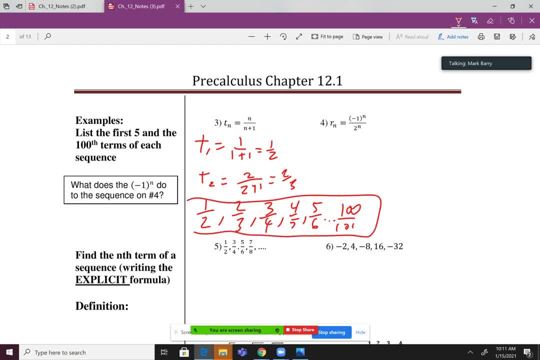 1 more than that, right? So at the point that you pick up a pattern and you can stop showing work, feel free to stop showing work, okay, I mean definitely this year. but even in a normal year where everyone is in class, my policy on showing work is: show work when you have to show work. 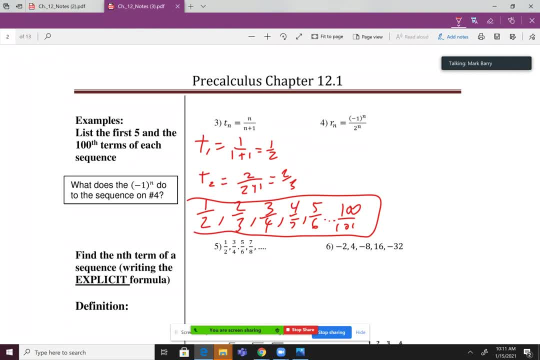 And if you don't have to show work, don't show work. If you can do it in your head, do it in your head. That's fine, okay, I understand. Okay, let's take on number 4 then. All right. so number 4, same idea. So r sub 1 is going to be negative 1 to the first power. 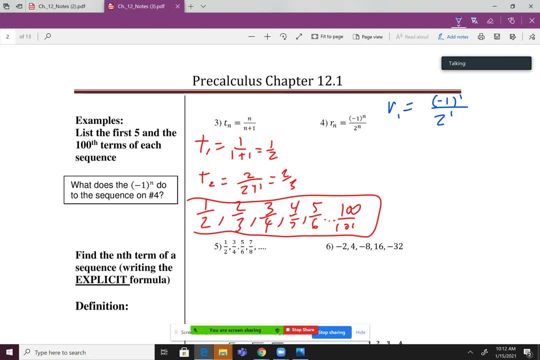 over 2 to the first power. So it's going to be negative 1 on top and a 2 on bottom. R sub 2, we get negative 1 on top squared over 2, squared R sub 3, negative 1 to the third power over 2 to the third power gives me negative 1 over 8.. 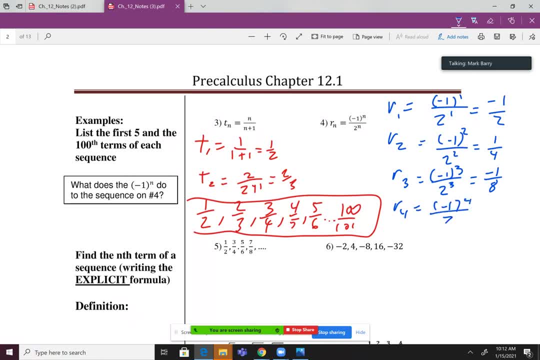 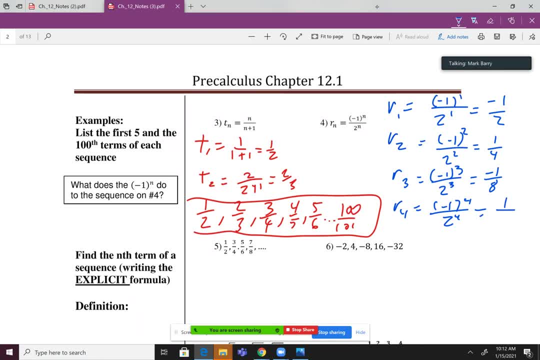 negative 1 to the fourth power is positive 1, and then 2 to the fourth power is 16.. All right, I'm going to pause there. I think I can build my list now, but I want to look at this question over here. So what does the negative 1 to the power of n? 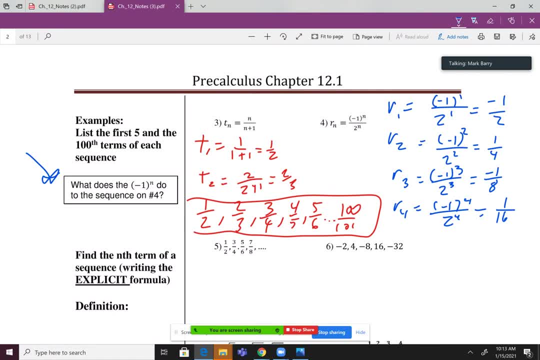 do to the sequence on number 4?. Okay, so let's have some participation here. You can type it in the chat or unmute yourself and say it. Can anybody tell me what that negative 1 to the power of n did to this sequence? Take a look at our terms in the sequence and tell me what effect. 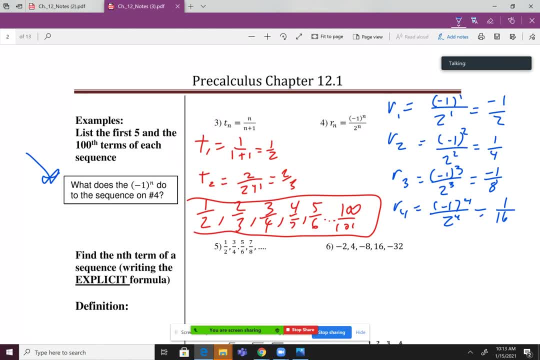 that that had on it? How did that negative 1 to the power of n affect the sequence? What are those? What are those numbers looking like My outputs And yes, Okay, and what effect did that have? Good, okay, and Kushi says the same thing that Logan's saying here in class. 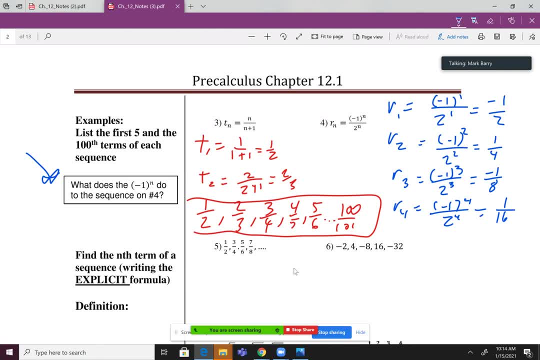 is that if it's odd, it's negative, and if it's an odd term, it's negative, If it's an even term, it's positive. Yes, it makes the sequence alternate positives and negatives. okay, Great observation there, Kushi, because that's going to help us going forward. 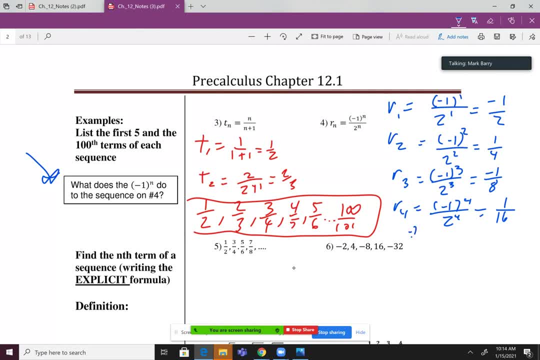 So my terms then, I would say, are: negative 1 half, and then positive 1 fourth, negative 1 eighth. positive 1 over 16, negative 1 over 32 would be the fifth term And then the sixth, or sorry. 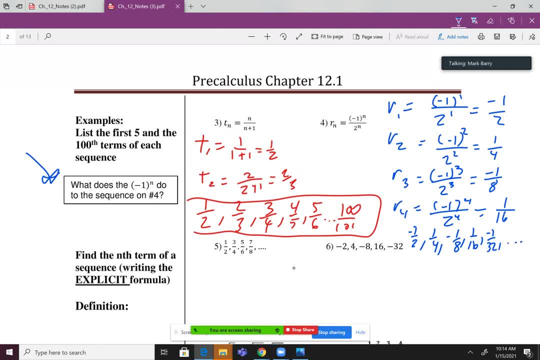 the hundredth term, I would say: well, since 100 is an even number and this is a comma right here, I know it's going to be a positive 1 up top, And then for the denominator, I would just put: 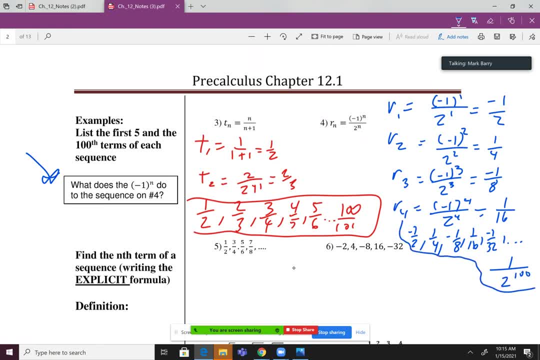 2 to the 100 power When you get these huge exponents and web assigns the same way with this, because that number is so big like your calculator can't even tell it to you. So if you get a huge exponent, just leave it like that, like 2 to the 100th power, okay. 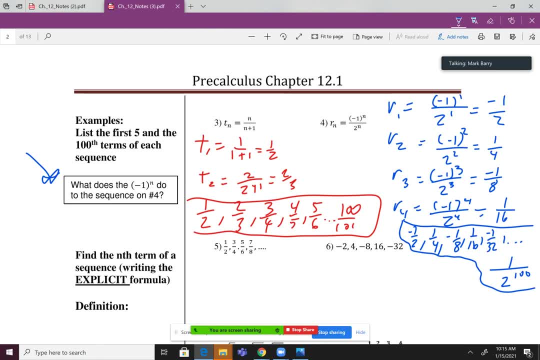 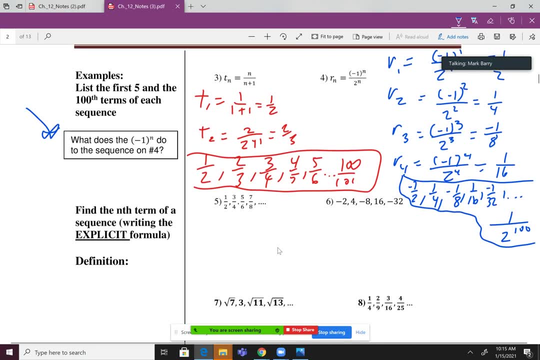 So that's that. So now we know if we have. so now we're going to kind of go the other way with this. You can see that on number 5 through 9 here. Now it's kind of the opposite, okay. So the question: 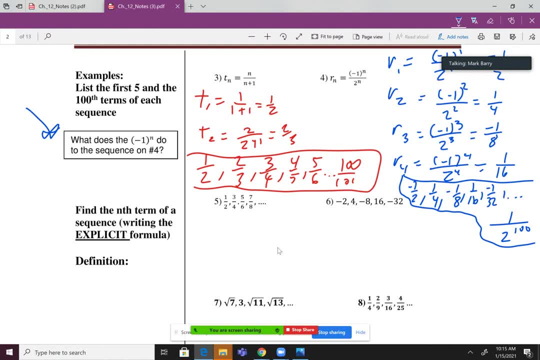 looks like our answers and the answer is going to be like the questions. okay, So we're trying to write a formula, But we have a tool now that we can use. If we have those alternating positives and negatives, could we use that negative 1 to the power of n trick that they used? Yes, we could, right. 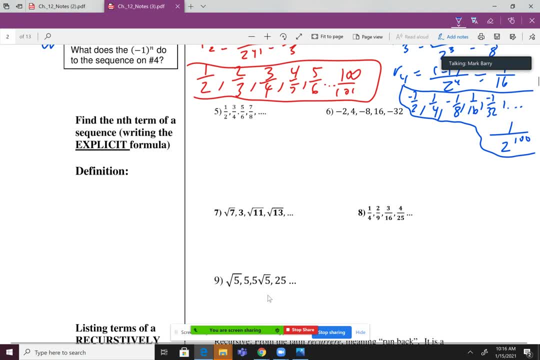 Okay, I'll give you a warning right now. Numbers 5 through 9 here: okay, These are the toughest questions that are in this whole section. all right, Students really struggle with these. So if you are watching us today and I'm going to really walk us through and help us on these- 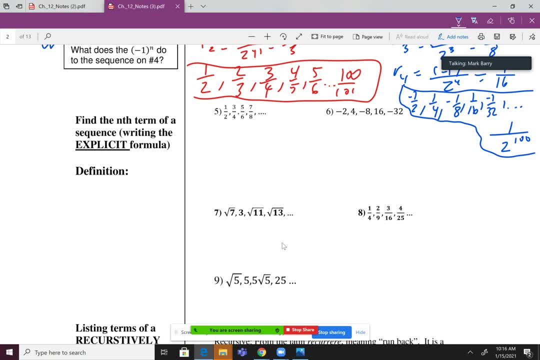 but if you're watching this today and like, oh man, this is going to be a hard one, this is so difficult, don't feel bad, you're not alone. okay, I will tell you that as we go through the next few sections in this unit, we learn a lot of tricks and formulas that help us. 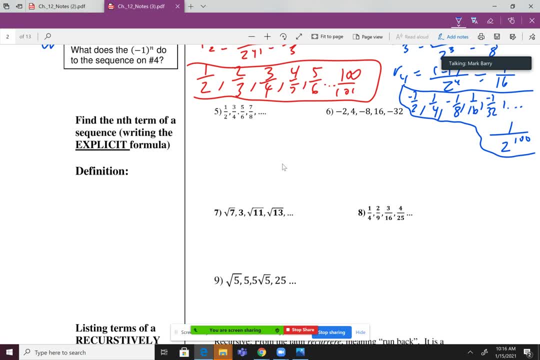 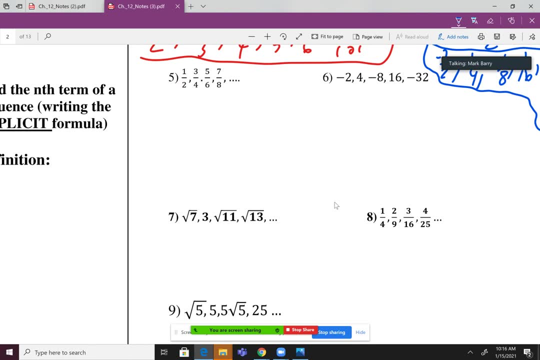 out with these, But for now it's going to be tricky, okay, So just follow along with me. All right, so number 5 here. all right, So number 5, we're trying to write a formula for these fractions here. Now, whenever the formula is all fractions, I would always just draw a big 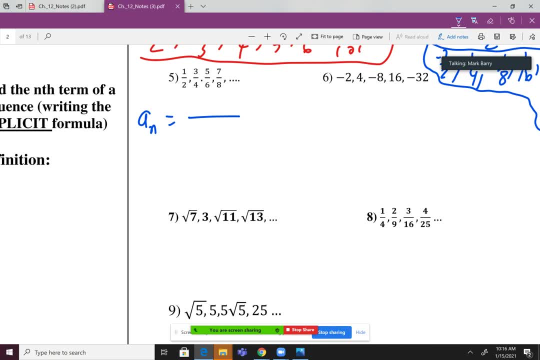 fraction. I would try to come up with a formula for the top and the bottom separately, okay, So just separate them in your mind. I'm actually going to start with the denominator on this one, because I think that's a little bit easier. So let's take a look at the denominator only How? 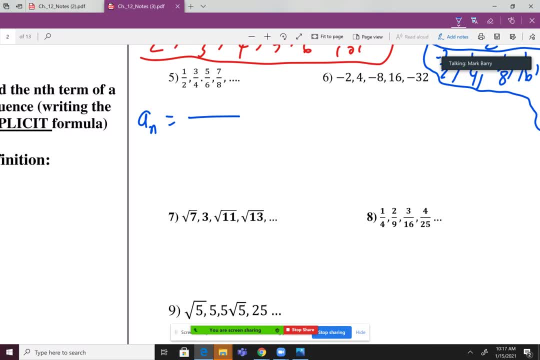 are we going to write a formula for that denominator. Well, what are the numbers in the denominator? 2,, 4,, 6,, 8,. okay, Multiply by 2 is correct, or? yeah, multiply by 2 is correct. 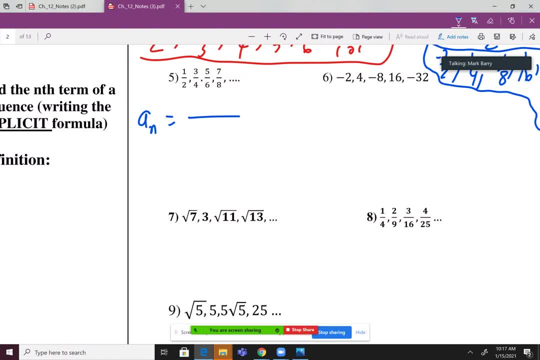 but let me tell you what most people put on this. Okay, whenever I kind of ask students this one, most students will write this on the denominator: They'll write n plus 2, okay, Now, that's not correct. I'll tell you right now. okay, But the. 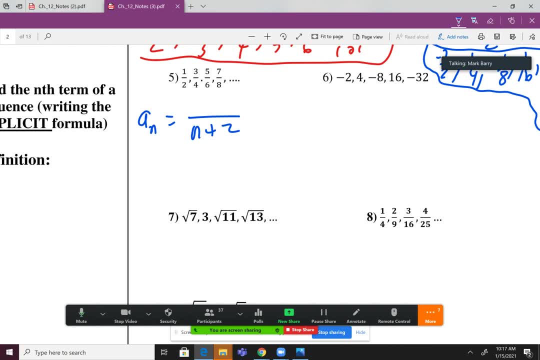 person who writes this: are they stupid? I'm going to say no, okay, They're not right, but they're not stupid either. Like they're saying: hey, Mr Berry, that denominator, the numbers, are increasing by 2 every time, right? So n plus 2, that makes sense. 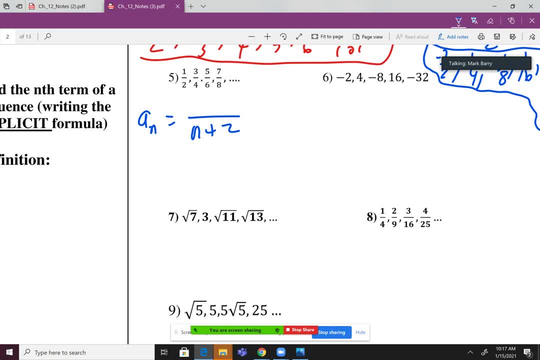 The great thing about these formulas is that we can check them. So let's plug in 1 and see if we get the correct denominator 1 plus 2, does that give me 2?? I have my first denominator, No, So I can. 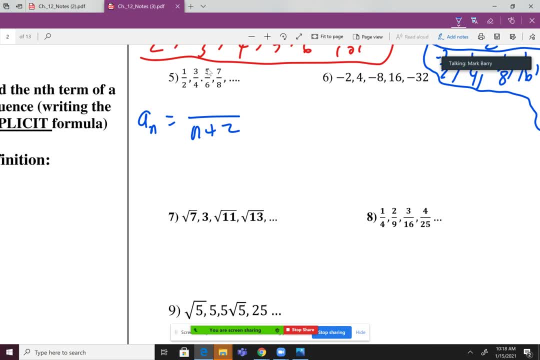 already tell it's wrong, correct? So good news: We just erased that. That's why they put pencils on erasers, or that's why they put this button on my stylus so I can erase that Now. Ethan said on the chat: 2n, Let's see if it works okay. 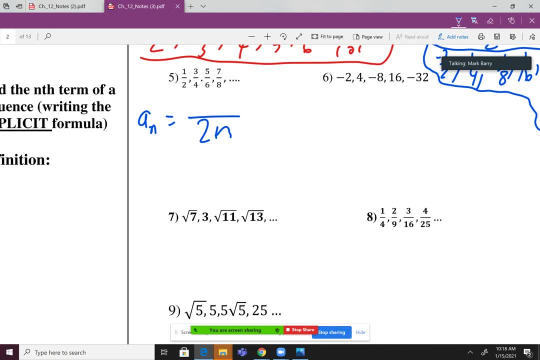 Sometimes you're not sure, but we can check it. So let's plug in: 1.. 2 times 1, does that give us our first denominator? Yes, 2 times 2,. does that give us our second denominator? Yes, 2 times 3, does that? 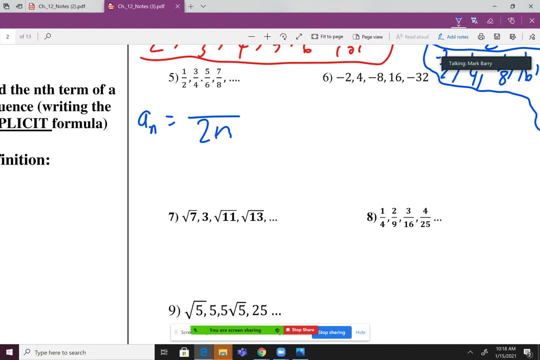 give us our third denominator, Yes, 2 times 4,, does that give us our fourth denominator, Yes, okay, So 2n is correct. Good job, Ethan. All right, what about the numerator? okay, The way I look at the. 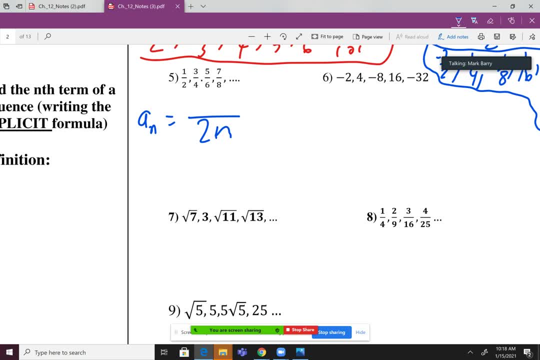 numerator. the numerator is always 1.. 1 less than the denominator. Look at every single individual numerator and you notice that it's 1 less than the denominator, correct? Well, if our denominator is 2n, what formula could we use? 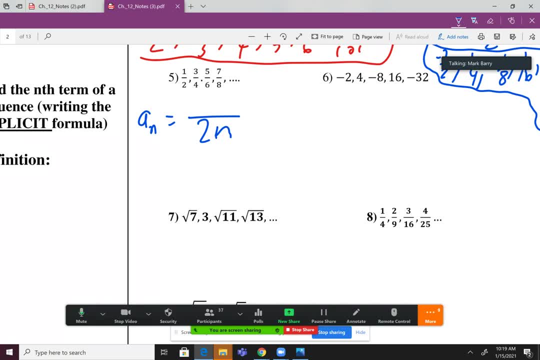 to come up with 1 less than 2n. 1 less than 2n Sounds good to me. Let's check it though, just to be sure, because these ones, I think, are so easy to check. So 2 times 1 minus 1, does that give us our first numerator? Gosh darn right, it does 2 times 2. 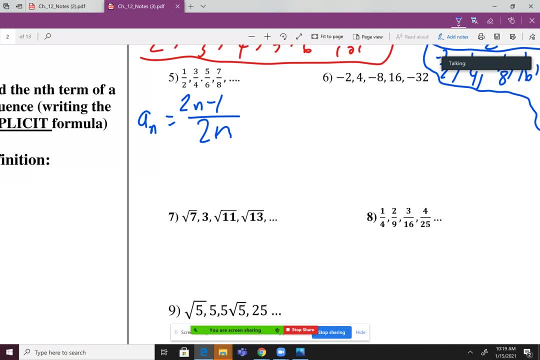 minus 1, does that give us our second denominator? Yes, 2 times 3 minus 1, does that give us our third denominator? Yes, 2 times 4 minus 1 gives us our fourth denominator: Yes, Nailed it okay. 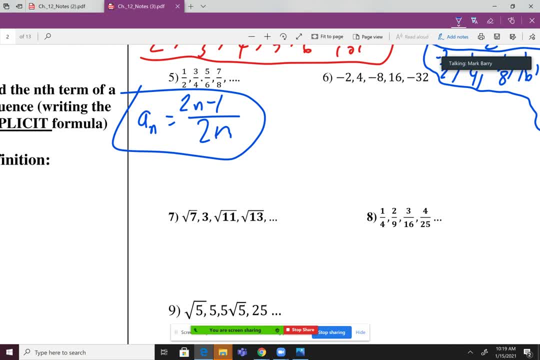 So there is some trial and error here, right? So if you get it wrong, just check it and adjust it right, like that's what this, i would say, is all about. okay, number six: first thing i notice on number six is we have those alternating positives and 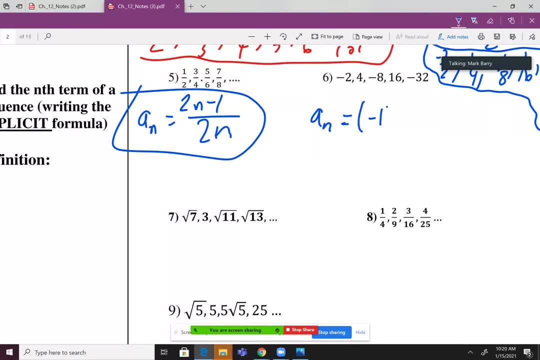 negatives again. right, so i'm going to go ahead and use that negative one to the power of n trick that i learned on number four for this. that's going to give me the alternating positives and negatives. this one's not a fraction, so i'm not going to draw a fraction line, so now i'm just 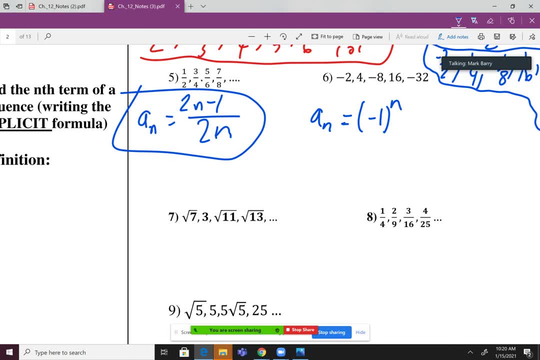 going to look at the numbers, so forget about the negatives now, since i already took care of that with my negative one to the n power. what are those numbers? 2, 4, 8, 16, 32, those numbers are significant to me. what are they? well, i would say that those are the powers of two, the powers of two, two to 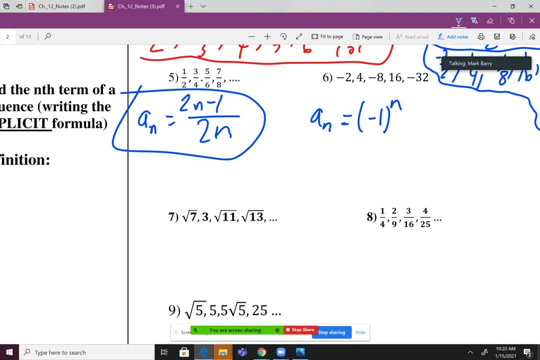 the first power, two to the second power, two to the third power is eight right. two to the fourth power is 16, and so i see this as times two to the power of n. so if i plug in, let's say i plug in three negative. one to the third power is negative. 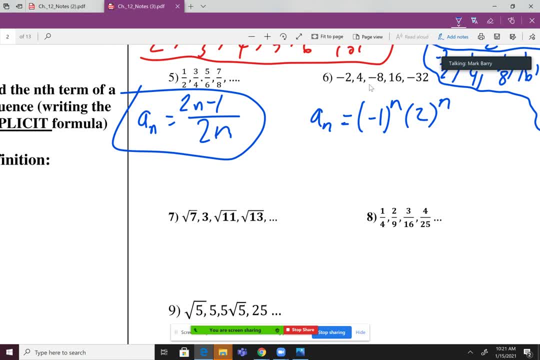 one times two to the third power is eight. so that gives me my third term of eight. the fourth power, negative one to the fourth power, is positive. one times two to the fourth power is 16. so this does work. so now some of you may be thinking, hey, mr berry, if i put negative two in parentheses and raise that to the power. 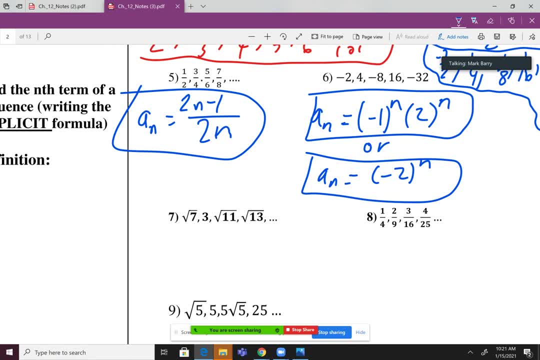 of n? wouldn't that also take care of the alternating positives and negatives, while still giving me all those numbers in that list? and to you i would say: yes, it does guess which one of these answers webassign says is correct. both of them, okay, that's something i 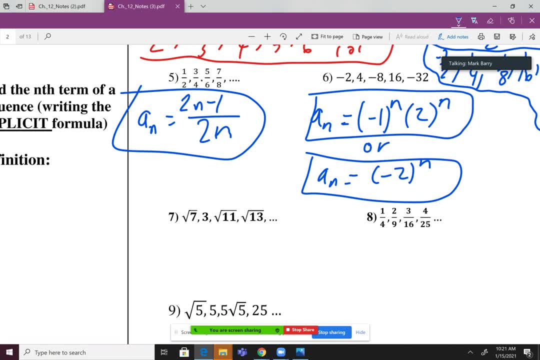 love so much about webassign. why i think it's it's such an awesome kind of platform- is that i would guess that their answer key says the bottom one. but even if your answer is different than their answer key, but it's still correct- it marks it as correct. so i think that. 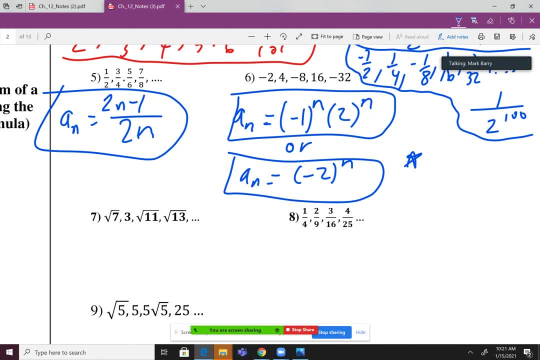 that's awesome. now what i'm going to note over here is that you cannot do this. if you did negative two to the n with no parentheses, that's actually incorrect. that sequence would actually be all negatives because of order of operations. you would do the two to the n parentheses and raise that to the power of n. so that's actually incorrect. 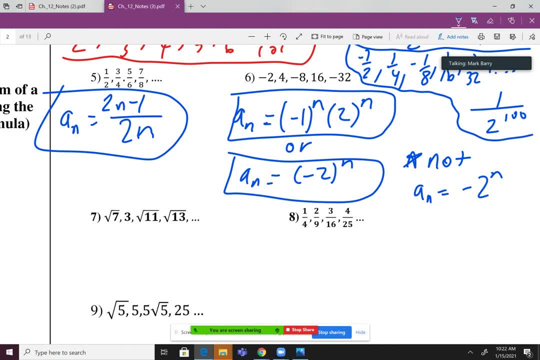 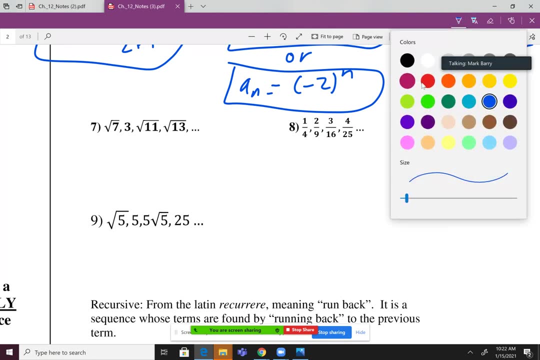 power first, which would be all positives, and then switch them negative, so it'd be all negative. so that's no good. gotta use those parentheses in this case. okay, all right, let's continue on. once again, we got three more here that are difficult. i i told you. 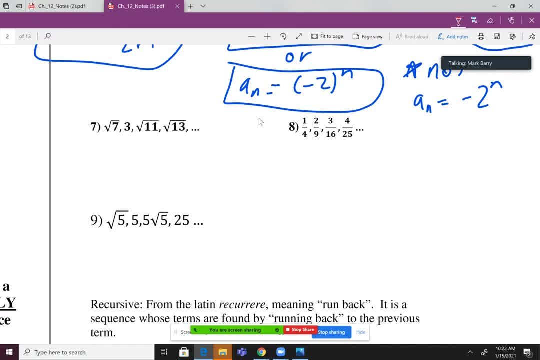 off the bat that these were like the most difficult ones that we're going to do. okay, oh, you know what? there's one at the end of the section that's. that's more difficult, but it's, it's similar. okay, so number seven: i'm looking at number seven and something's popping out at me. 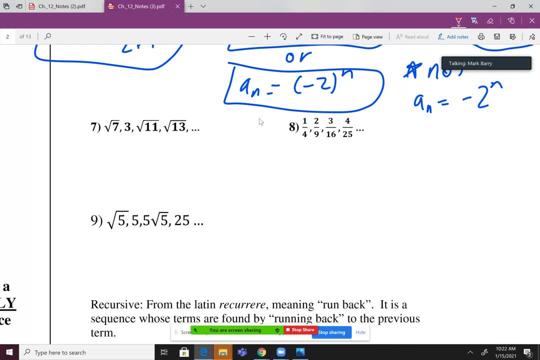 something i don't like here. okay, one of these terms is not like the others. do you guys notice that? which term is not like the others? the three, right, that's. that's sticking out like a sore thumb. like what is that three doing there? well, is there a way that we could rewrite three? 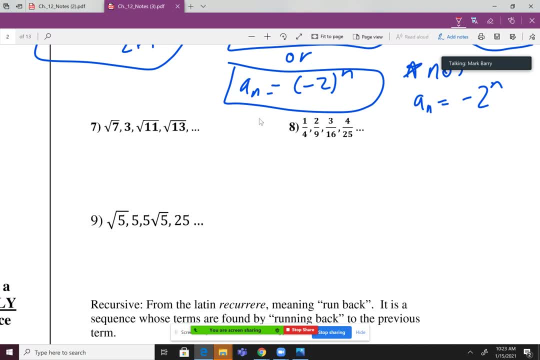 that would make it look more like all the other ones. i think there is um, not three squared. you're on the right track there, brenda. i'm gonna write it as rad nine. did i really change it? no, is rad nine the same thing as three? yes, so why do i want that written? 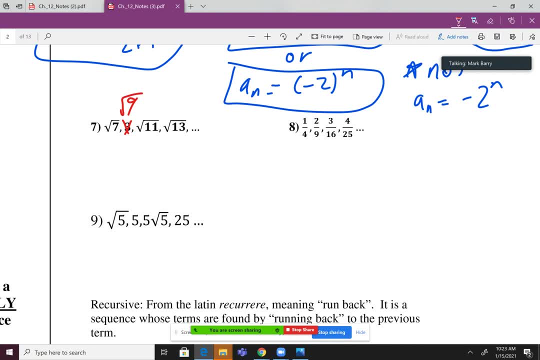 as rad nine. well, it's like apples to apples comparison. now right, like we're looking at everything inside of a radical and we're looking at everything inside of a radical. so now i think, and and actually, if i look inside of those radicals now, it makes a pretty good. 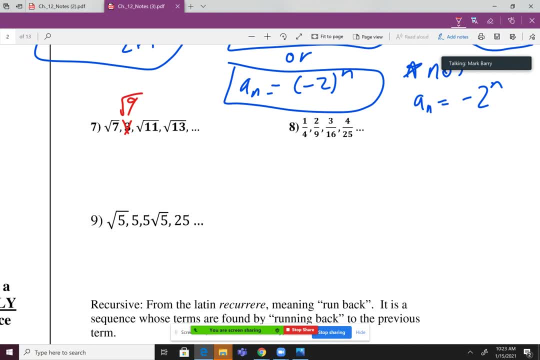 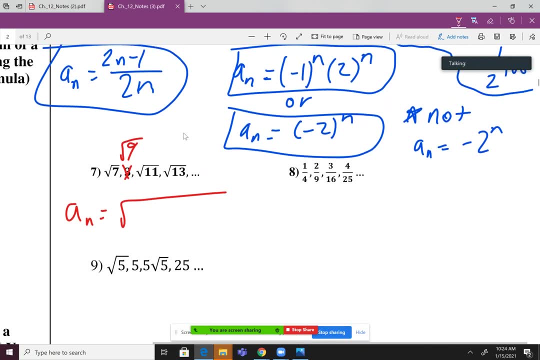 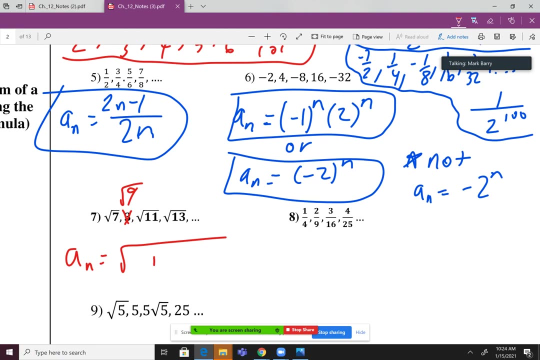 pattern. right, it's that plus two pattern. you know what i'm saying, so i'm gonna write my formula now. a sub n equals. i'll draw a big radical, as we saw on number five. when you have that increasing by two pattern, it's going to be something with 2n, okay, which is also the name of our principle, right- 2n. 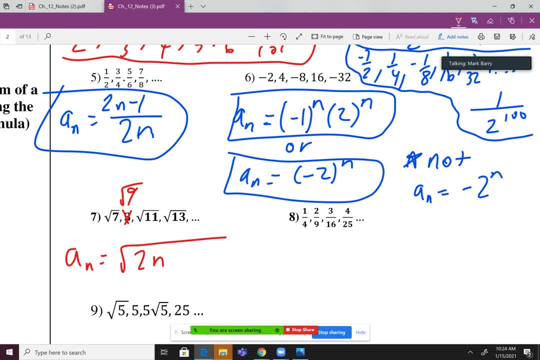 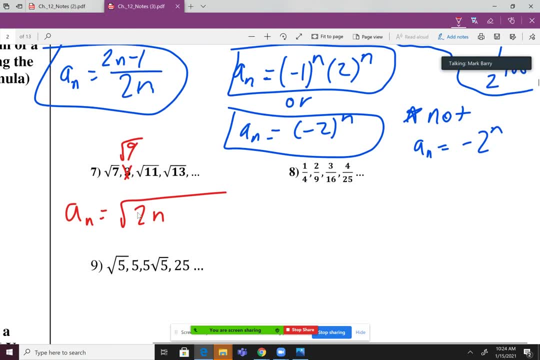 dr 2n. now it's not just going to be 2n here on number seven, but it's going to have something to do with 2n. so my point is: whenever you see that plus two pattern, think about 2n if you see like a plus three, 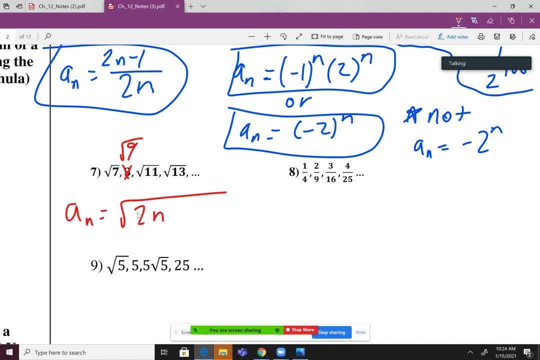 pattern. think about 3n. you know what i'm saying. so if i just leave it as 2n, if i plug in one right now, i'm not going to get seven, right, i'm going to get two. so what would i need to add to this? 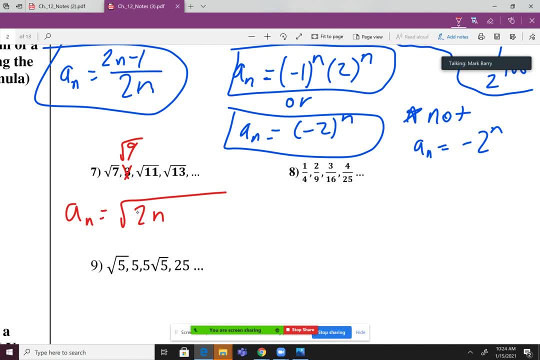 so when i plug in one, i get seven and i'm going to get two. so i'm going to get two and i'm going to get seven. well, when you ask it like that, it's got to be five, right. don't take my word for it, though. test it two times. one plus five gives you seven inside of a radical. 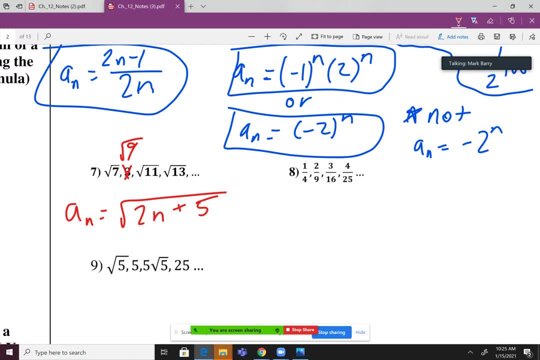 doesn't it? two times two plus five gives you nine inside of a radical, doesn't it? two times three plus five gives you 11 inside of a radical, doesn't it? and two times four plus five gives you 13 inside of a radical, doesn't it? 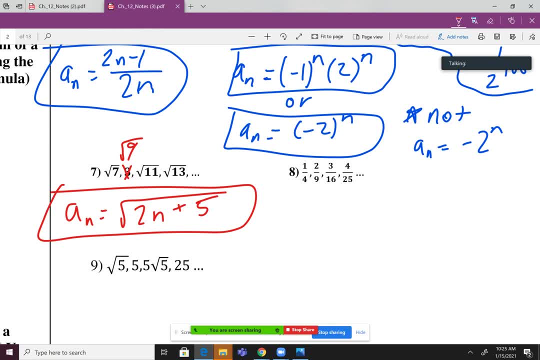 guess it does all right onward. number eight: we got another fraction for number eight, so i'm going to draw a big fraction line. i'm going to tackle the numerator and denominator separately. numerator first. i think the numerator is simpler. on this one, i think the numerator is actually very simple. 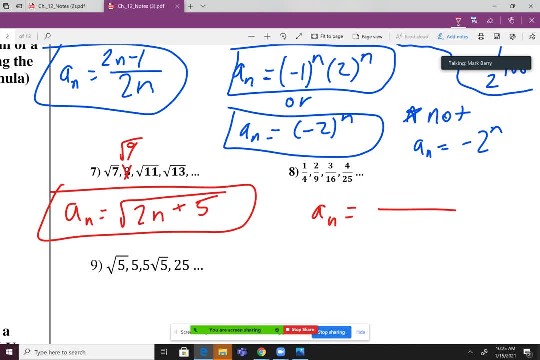 it is very simple: it is changing right. so if there's ever one where, like, the number is staying the same the whole time, like just put that number. but if it is changing we do need a variable. i would say the numerator is just n right, like, whatever number we're on, that's our number. so 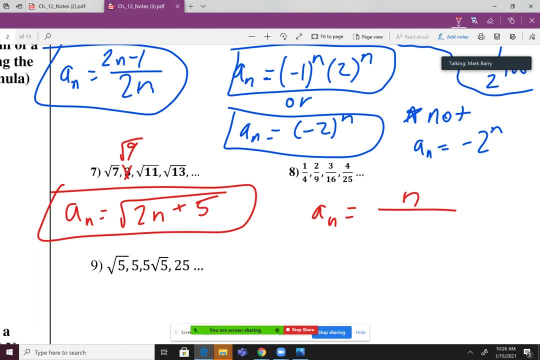 for the first term it's one. for the second term it's two. for the third term it's three. for the fourth term it's four. denominator is a little more tricky here, but i do notice something about those four numbers in the denominator. are those four numbers in the denominator? are they the same number or are they? 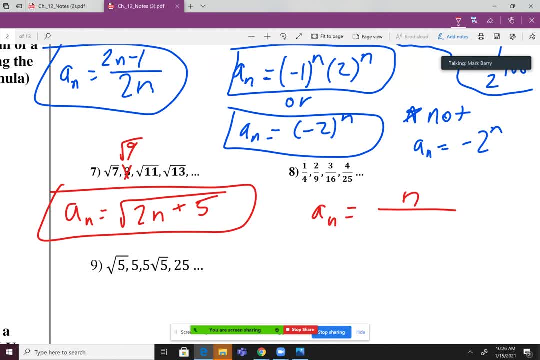 denominator: special numbers, i think. so they're special to me. well, all numbers are special to me, but these numbers are especially special. these are perfect squares, correct, perfect squares? for sure, okay, but it's kind of the wrong perfect square like the like. the first one isn't one squared, the first one's two squared. the second one is three squared, the third one is four. 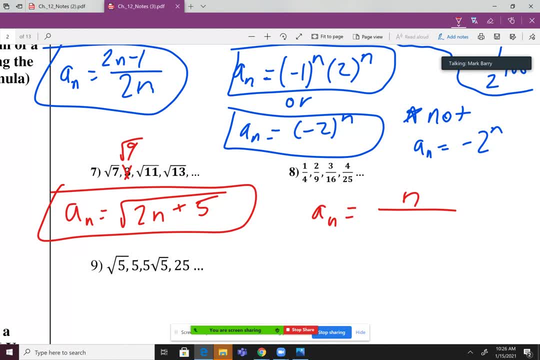 squared. you know what i'm saying. so i need to add one to the denominator, and then i'm going to put it together, and then i'm going to one before i square it. okay, because if i square it right away, i'm going to get the wrong number. 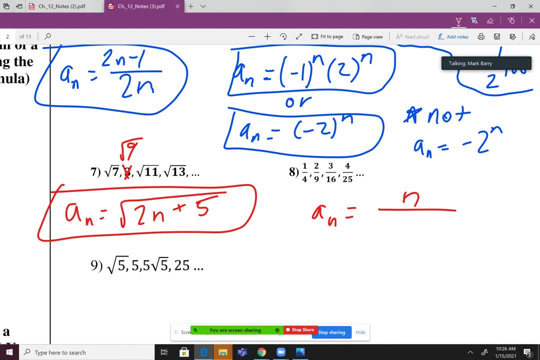 so i need to add one before i square it. i've seen three people in the chat now get the correct numerator, sorry denominator- here, which is n, plus one in parentheses, which is saying: add one before you square it. very good, shout out to you: uh, achie Lan, Tammy and Adam. alright, good stuff. 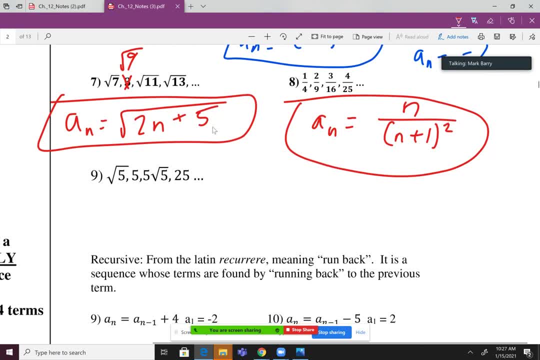 alright, number nine: very tricky as well. okay, like i said, if this is seeming difficult, it is okay, but remember also it will get easier. okay, so number nine. what do i notice? so the first term is rad 5, the second term is 5 and number six: what do i notice? 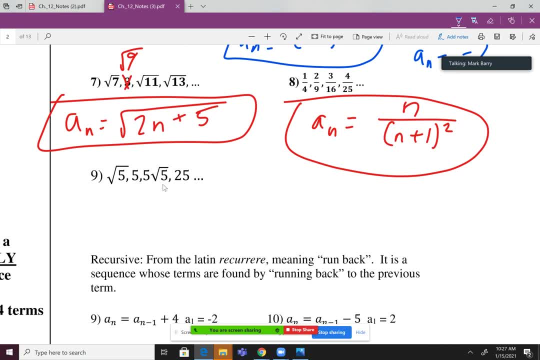 10 is negative and 19 is negative, then it gets 5, rad 5 and then 25.. The thing I noticed right off the bat is that rad 5 squared is 5, right Rad 5 squared equals 5.. So my initial instinct here would be: if I take rad 5 and raise, 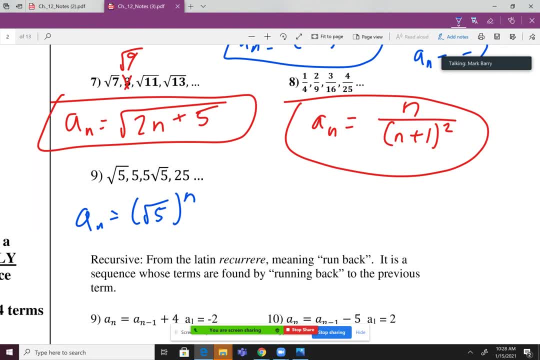 it to the power of n. I know that that's going to work, for the first two terms at least, because I know rad 5 to the first power is rad 5, right, Anything, the first power is just itself. I also know that rad 5 squared is 5, so I know it works for those. So now the question is: does that work? 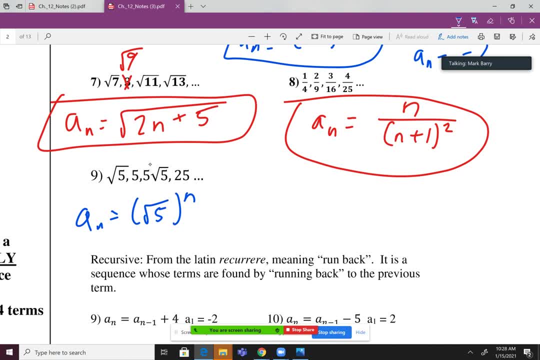 for 3 and 4, right? Let's check it out. What's a sub 3?? Well, according to my formula, that would be rad 5 to the third power. I see that as rad 5 times rad, 5 times rad 5, right. 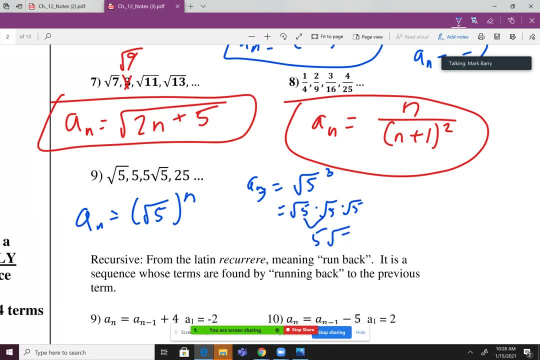 Well, if I multiply rad 5 times rad 5, that would just be a regular 5.. So it would be 5 rad 5, which checks out right. That's what I wanted. I'm feeling pretty good about my formula at this point. Let's check out the fourth power. 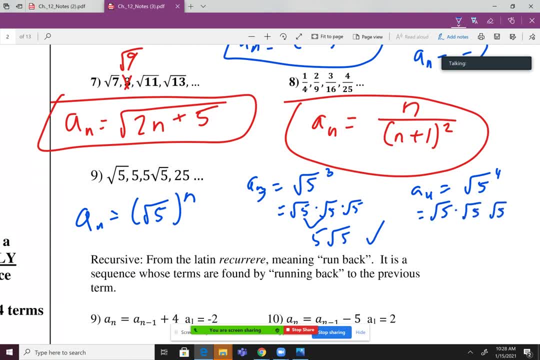 though. Well, if I pair these guys up, it's going to give me 25 all day, every day. If you wanted to get really savage with this formula, you could write it like this: 5 to the power of n over 2.. 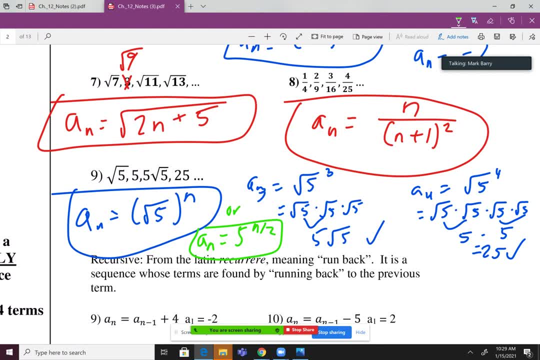 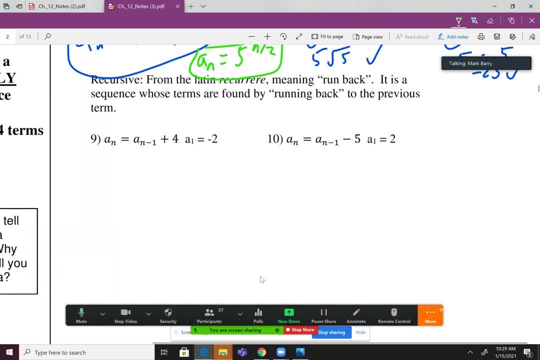 If you're into fractional exponents, which I certainly am, all right. that's a little bonus for you. You can check that out later on your own time, but I'd say the blue one is sufficient for that, okay. Okay, let's keep it going here. Now we're actually going to learn about a new 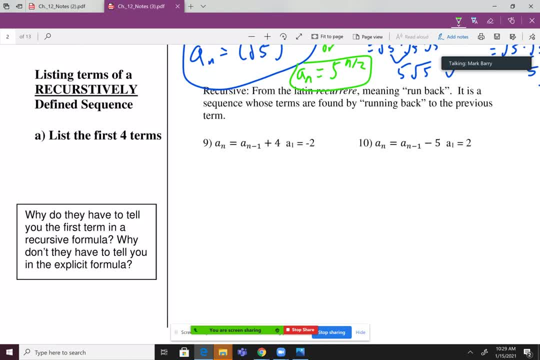 way to write a sequence now and that's called a recursive sequence. okay, Recursive sequence. So I said that previous. those last five questions we did were the hardest ones, So these ones are easier. okay, It's a little complicated to understand these. 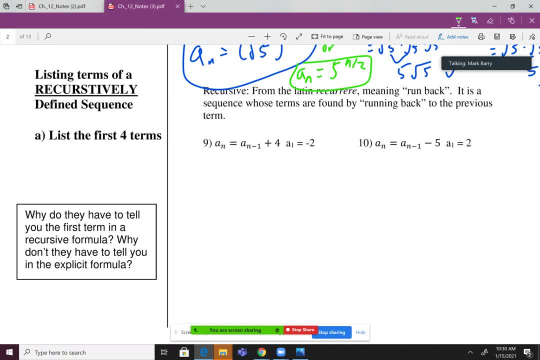 but once you understand, these are actually easier. okay, How do I know that these are recursive? Whenever you see like the sub n minus 1 here, that's my indicator that this is recursive. These ones: each term in the sequence is based on the previous term. okay, Now what's kind of unique about these ones is that 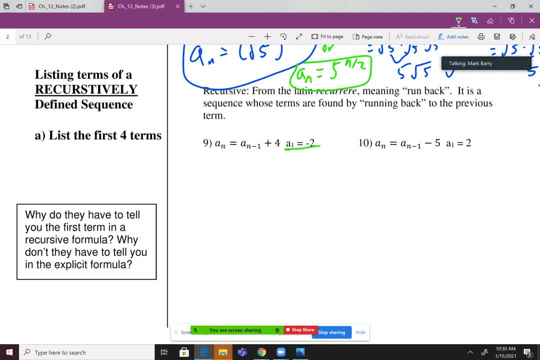 you'll notice, they actually gave you the first term right. So on all our previous ones, when we're trying to find the first four terms, we had to find the first term on our own. In this case, they told me the first term. They said, hey, find the first four terms. but guess what? Here's. 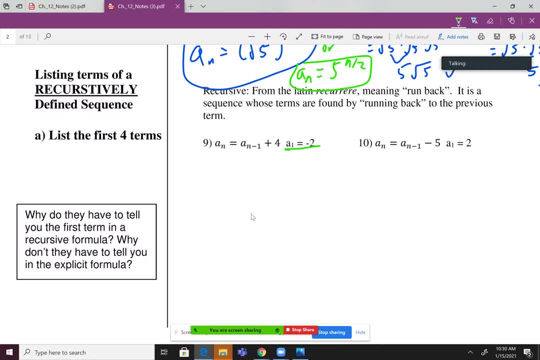 the first term. It's negative 2.. Well, if they already told me the first term, I would say the next one I should try to find is the second term. right, I don't need to find the first term because they already told me. So I'm saying n is 2,, right? So if n is 2, then n minus 1 would actually be 1.. 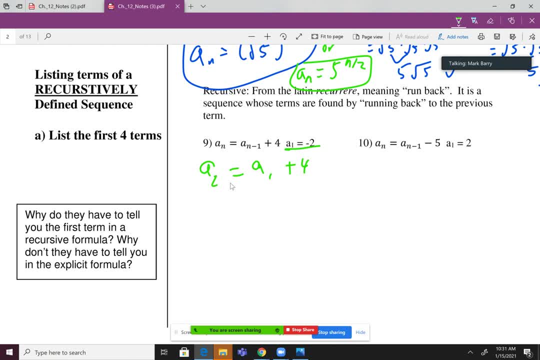 So they're saying: a sub n minus 1 is negative 2.. So 2 here equals a sub 1 plus 4.. Well, we actually know what a sub 1 is. A sub 1 is negative 2, correct. So our second term is 2.. I could do that again, and this is like the complicated way to do. 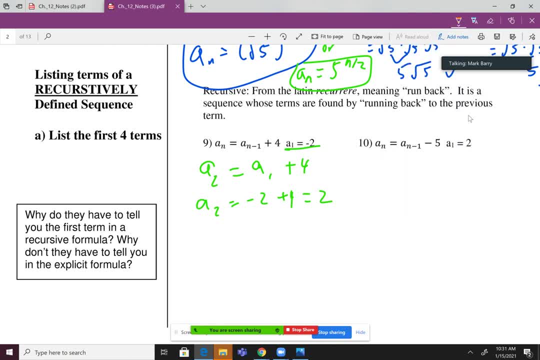 it. but can I tell you guys just the easier way to understand these sequences? Okay, I'll take that as a yes. Whenever you see this. a sub n minus 1, you're going to have to find the first term. I want you guys to just read that as the previous term, the previous term in the sequence. 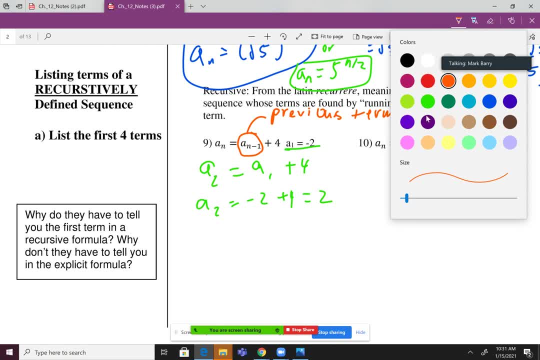 So, for all of these recursive formulas, they're going to tell you, take the previous term and do something to it. What are we doing? in this case? Adding 4.. That's it. So I'm going to stop showing my work. I'm going to stop showing my work. I'm going to stop showing my work. I'm going to. 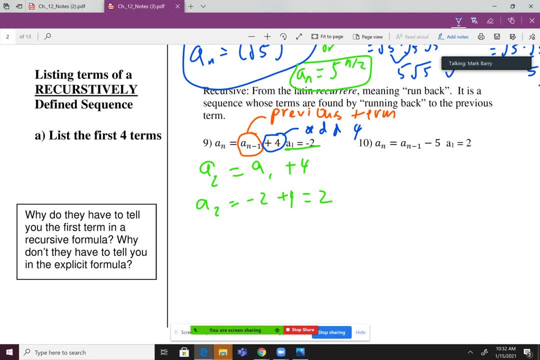 start showing my sequence. Where does my sequence start? It starts at negative 2.. How do I know it starts at negative 2? It was given correct. They told me A lot of people. they always start this with the second term because that's the first term that they found. and people are like: 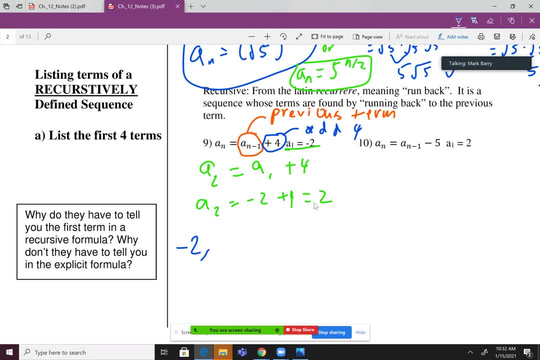 narcissistic and they're like: oh, that's the first term I found, so that must be the first term. No, no, no, Don't be a narcissist, It's not the first term you found, It's the first term. 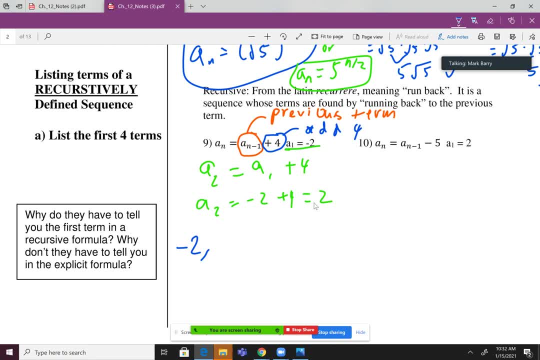 First term, a sub 1.. For these it's given Negative 2.. Now to find the next term. this says: take the previous term and add 4.. So I take negative 2, add 4.. Take 2, add 4.. Previous. 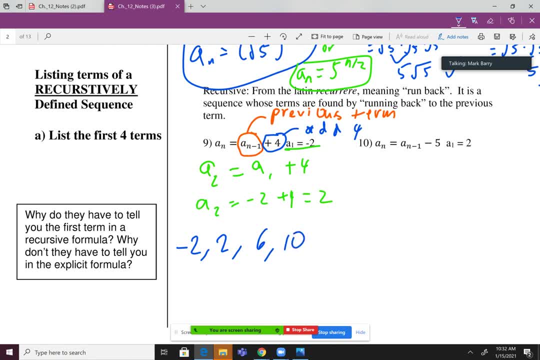 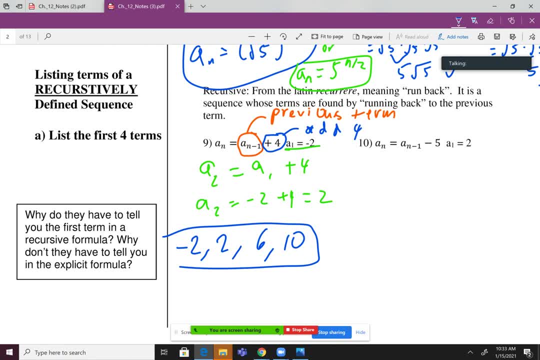 it. Why do they have to tell you the first term? Well, if you told me to do a plus 4 pattern and you instead told me to start at 50, it would be a totally different sequence, correct? So each term is based on the previous term, so you have to tell me where to start. 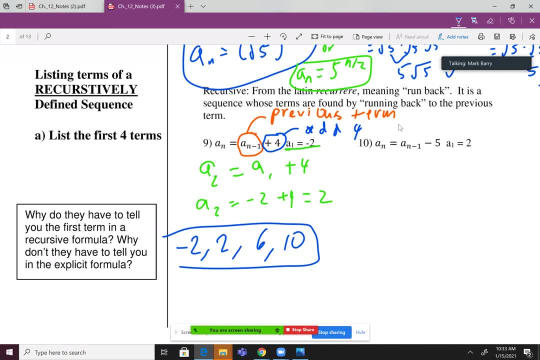 All right. so same idea on number 10.. We're starting off at 2.. How do I know we're starting off at 2? They literally told me First term's a given. Then to find the next term, it says take the previous term and add 4.. So that's it. 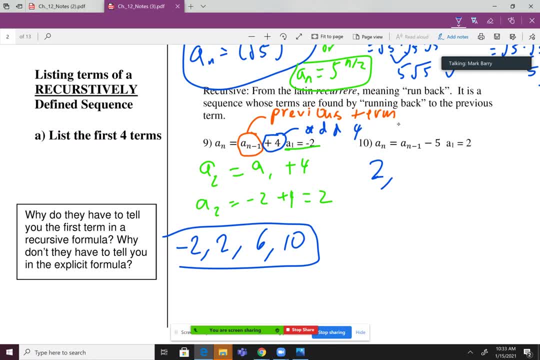 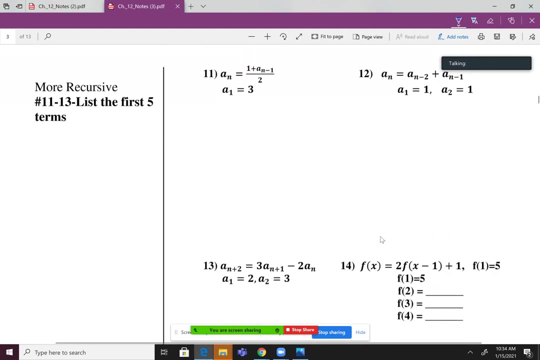 And each subsequent term I just keep subtracting 5.. So minus 5.. Minus 5., Minus 5.. All right, Not too bad right, Let's keep going. All right, so now our sequence gets a little bit more complicated here on number 11.. I'm 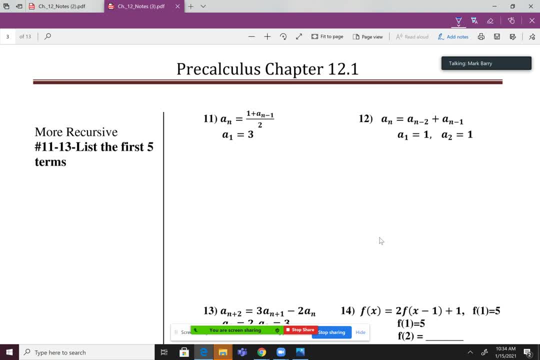 actually going to show my work on this one because it is a little bit more complicated. So we already know what a sub 1 is: It's 3.. So a sub 2 would be 1 plus the previous term divided by 2.. So whenever you see that a sub n minus 1, that just means plug in the previous 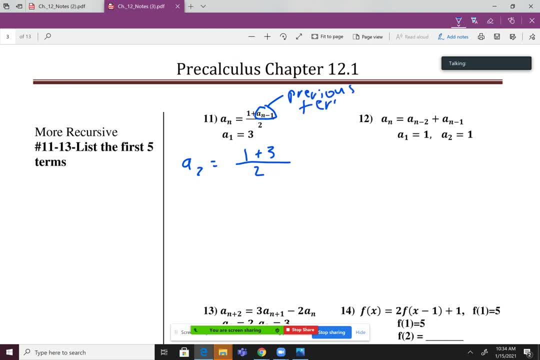 term. whatever it is, It will be changing along the way. So now I got a sub 2 is 2.. A sub 3 then is 1 plus the previous term over 2.. However, now the previous term is 2.. 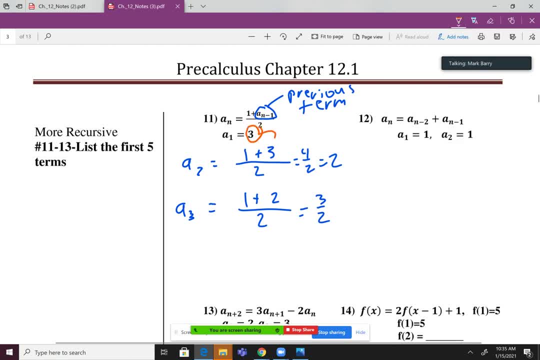 So where am I getting these numbers? once again, a sub 1 goes right there, and then this answer goes right there. That position in the top right of this particular fraction is where I'm plugging in the previous term. So that's where this 3 over 2 is going to go in my next round here. 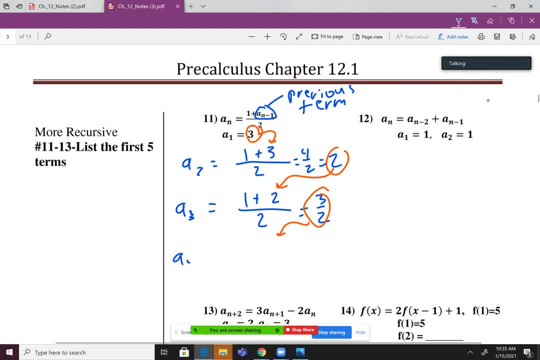 So for a sub 4, 1 plus 3 over 2, plugging in my previous term there over 2.. I'm going to add those fractions. Of course we need common denominator there, so I'm going to turn that into 2 over 2.. 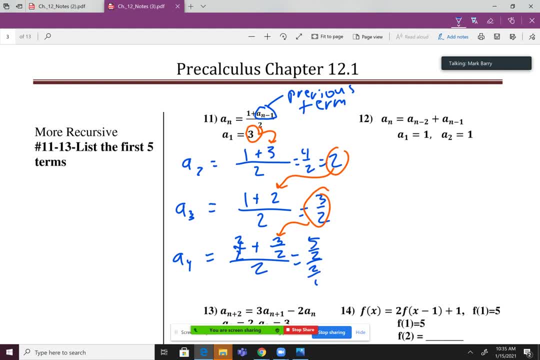 So we get 5 over 2 over 2 over 1.. Multiply by the reciprocal: We get 5 over 4.. So my list of my first four terms would be: 3, 2, 3 over 2.. 3 over 2, 5 over 4.. 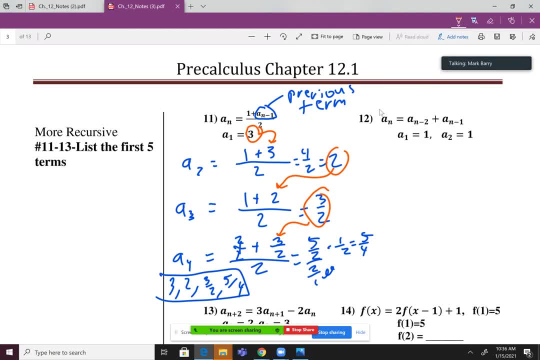 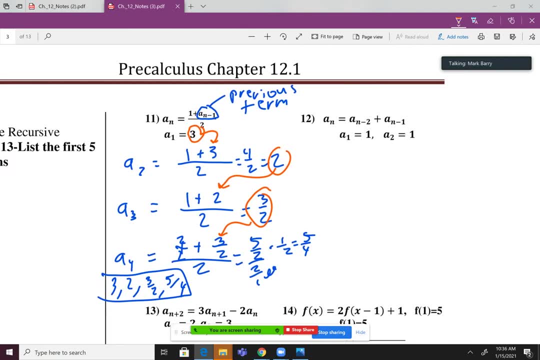 All right, we've got time for one more problem, and it's one of my favorites: number 12.. Number 12, you can see what they did. that's a little bit different here is they told me the first two terms, right. 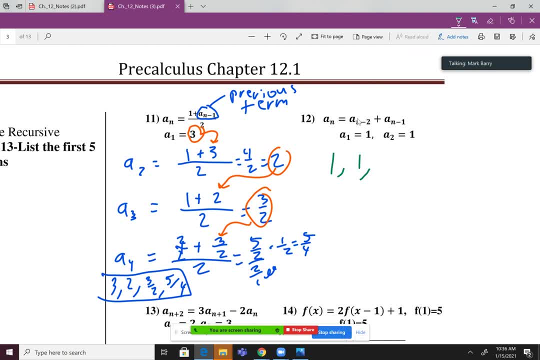 Well, what does this mean? over here, a sub n equals a sub n minus 2 plus a sub n minus 1.. Well, to me that means, if I want a sub 3, I would have to add a sub 1 and a sub 2.. 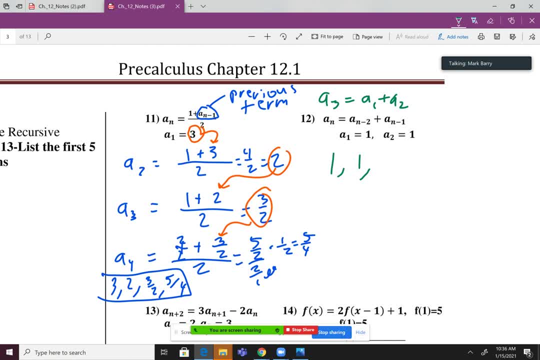 So this to me suggests- and this is why they gave me two terms to start- each term is the sum of the previous two terms. So 1 plus 1 then gives me 2.. My fourth term is 1 plus 2.. 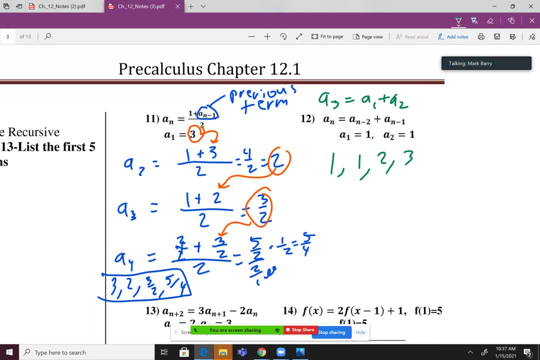 The previous two terms is going to give me 3.. I'm going to keep going with this. I know I've been doing 4, but I want to keep going. So 2 plus 3 gives me 5.. 3 plus 5 gives me 8.. 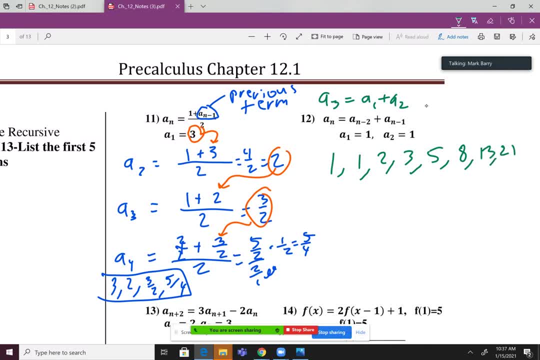 5 plus 8 gives me 13.. 21,, 34,, 55, etc. This is actually a famous sequence. This sequence actually appears in nature All the time. I'll show you guys a video, a quick video, about this sequence on Tuesday. 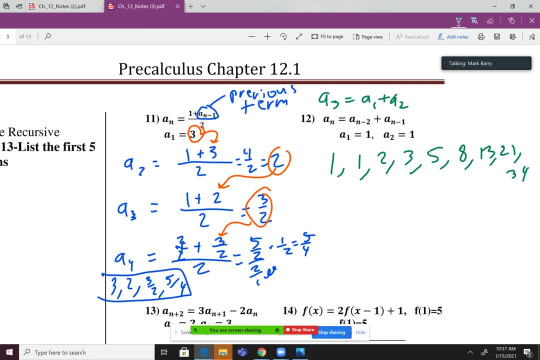 the next day we meet, since we have Monday off. But yeah, does anybody know the name of this famous sequence? It's named after an Italian mathematician who did a lot of work with it. It is not to be confused with the Fettuccine sequence. 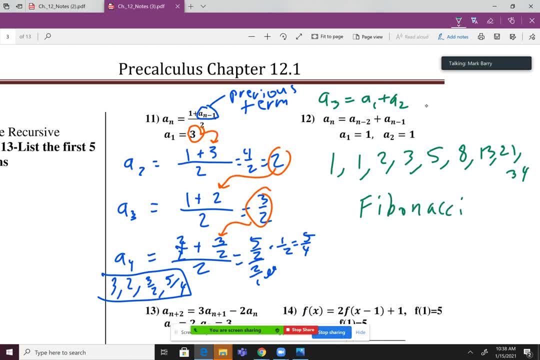 It's the fib. Go ahead and write this down. Fibonacci sequence. Not something that's really going to show up on a test here or anything, but just an interesting thing for you to know, This famous sequence. It is often I do hear it referenced in like I don't know pop culture or whatever. 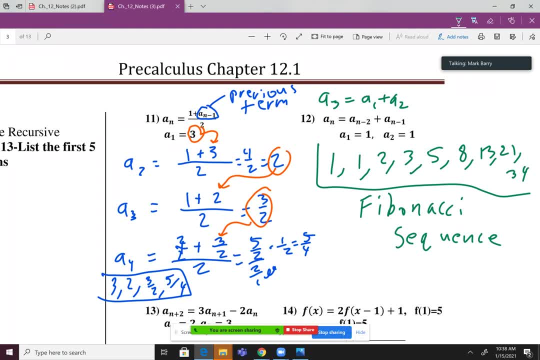 The Fibonacci sequence, So it's a good thing for you to be familiar with. It's this list of numbers, okay: 1, 1,, 2,, 3,, 5,, 8,, 13,, 21,, 34, and so on, okay. 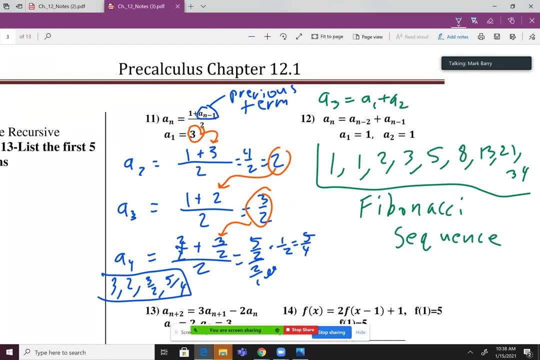 Like I said, we'll watch a video, a quick video about that, on Tuesday, But For today, I don't know if you guys knew this about me, but I like to throw some memes in there, right? So I happen to have a Fibonacci sequence meme. 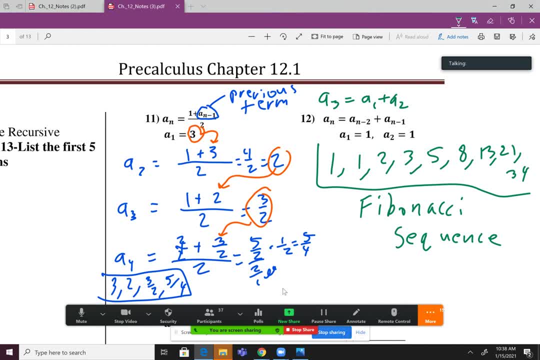 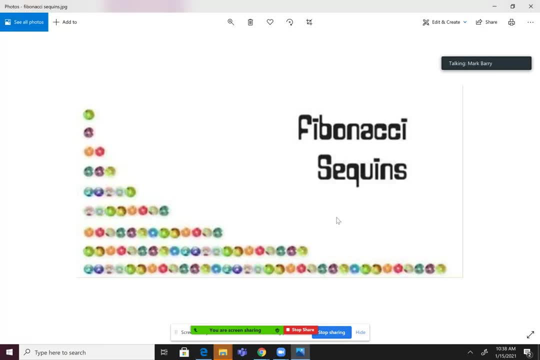 So let's check that out. So you've heard of the Fibonacci sequence, right? How about some Fibonacci sequins? Look at the numbers of the sequins: 1, 1, 2, 3 sequins, 5 sequins, 8 sequins, 13 sequins. 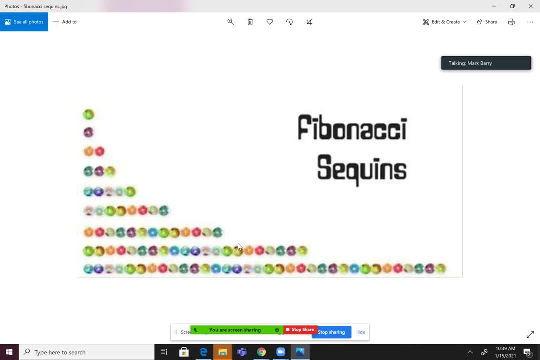 Get it. It's funny, Okay, cool. So that'll about wrap it up for our notes for today. So remember, I'm going to post this video of what we did today because I did a pretty good job this period on YouTube. 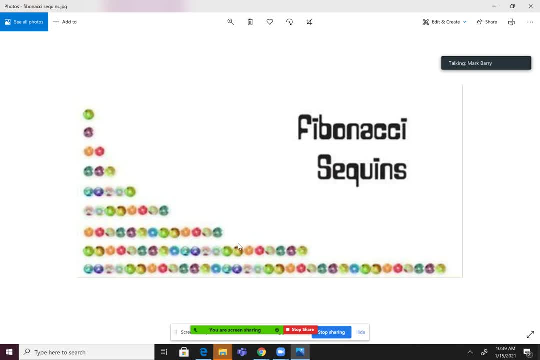 and I'll post that on Schoology And then I'll make another video. that'll be the rest of the section. okay, I would like you guys to do the rest of the section over the weekend and we can get going on our website on Tuesday when we get back. all right, 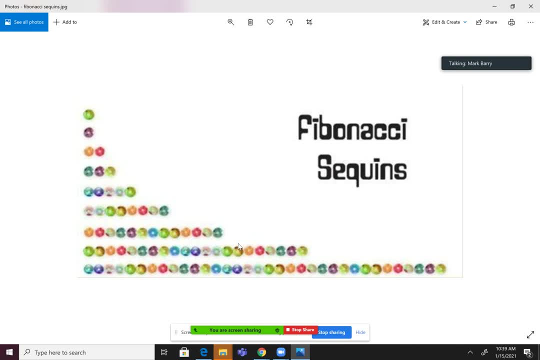 So we do have a little bit of homework over the weekend. just the rest of the section, with the help of my notes video that'll be posted this afternoon So you can do it anytime this weekend. I think it'll be 15 minutes or less, I'm pretty sure. 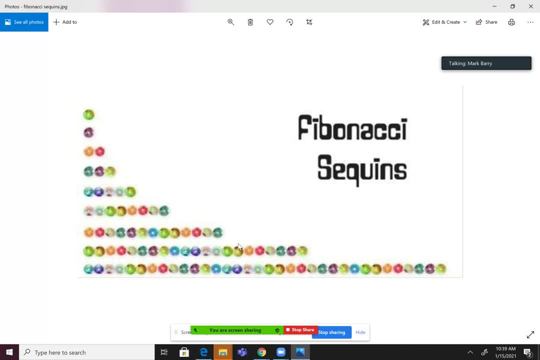 to get the rest of it done. I haven't made it yet, so YOLO. All right, I think that's all I got, So stick around a couple of minutes for questions, but if you don't have any, then we will see you on Tuesday. 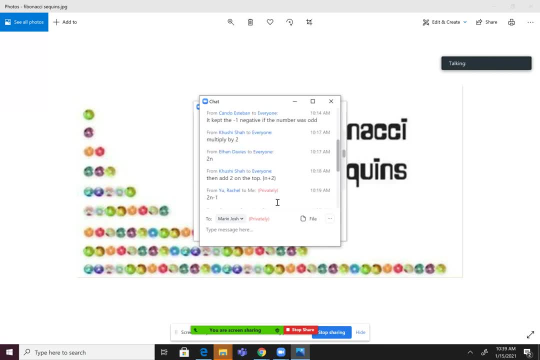 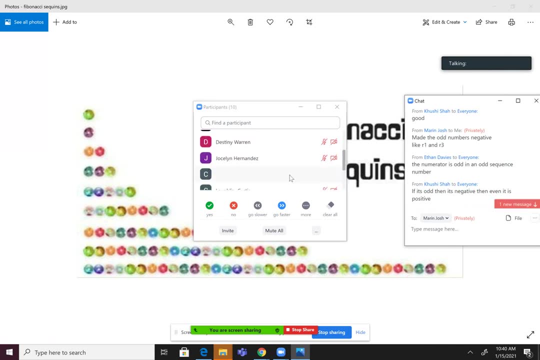 Okay, Bye, You're welcome. 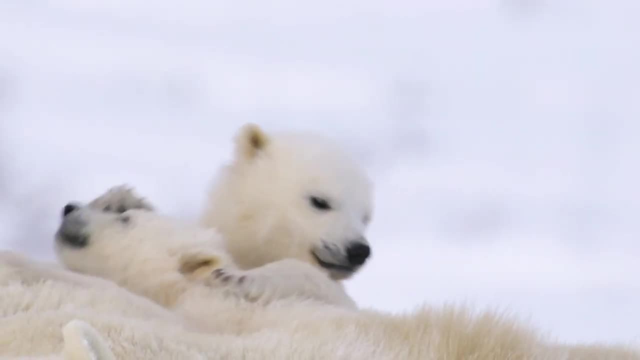 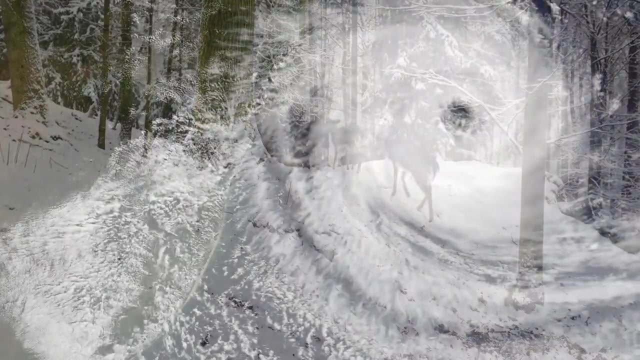 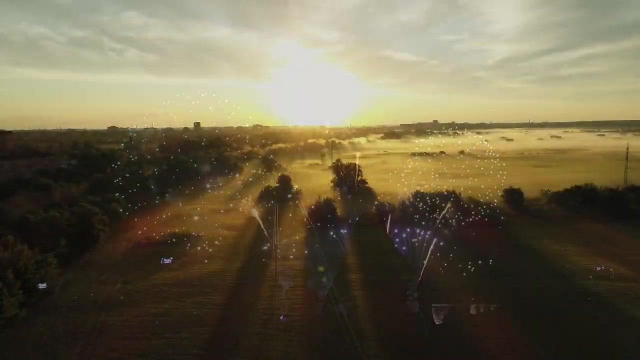 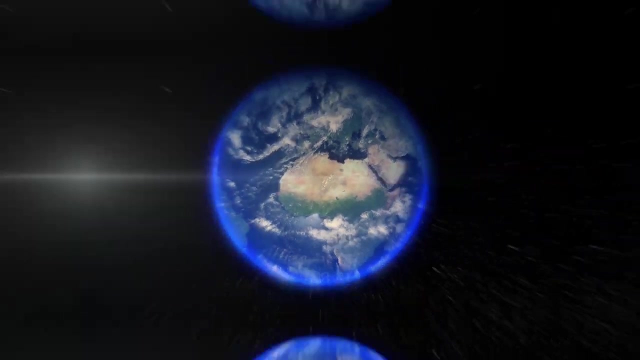 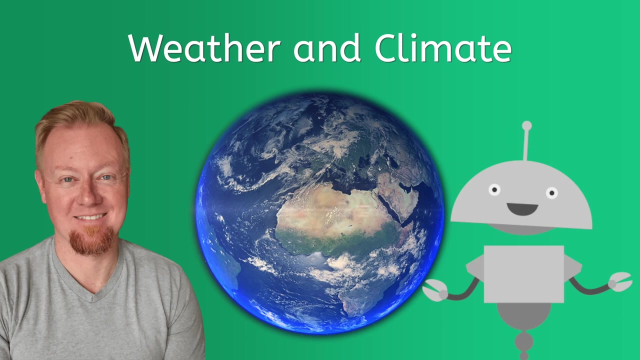 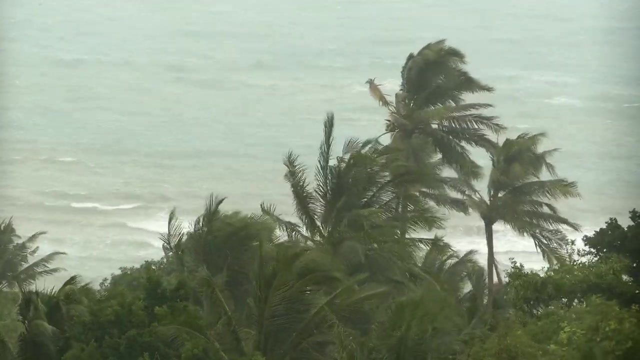 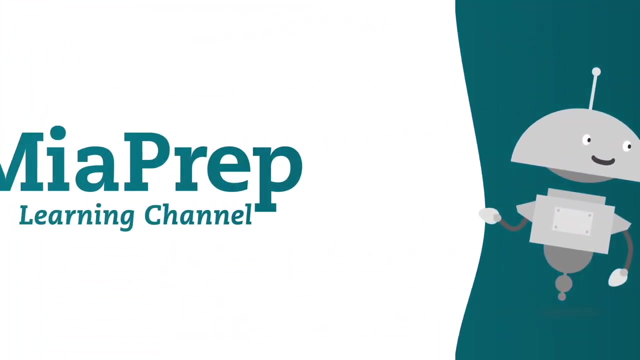 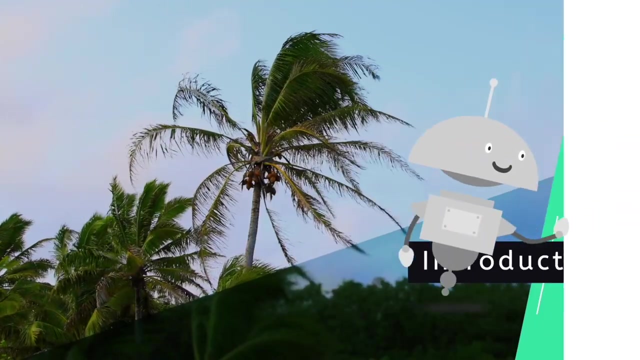 Welcome back Explorers. It's Brian here with you, and today we'll continue getting to know the Earth by studying its day-to-day and long-term trends. I hope you're ready for another adventure, because this one could get a little windy. 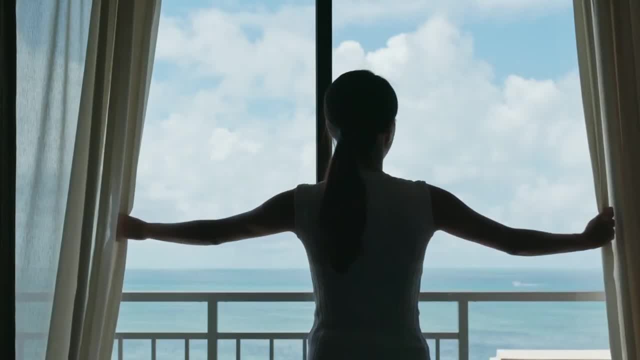 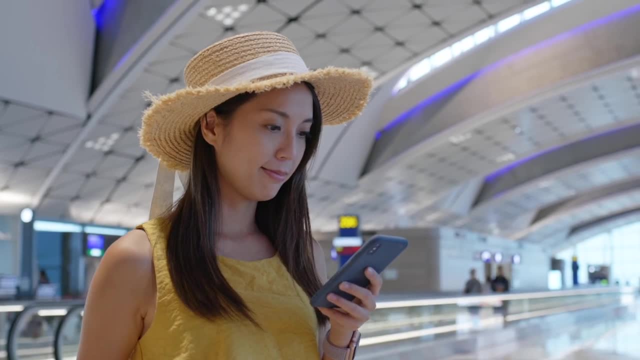 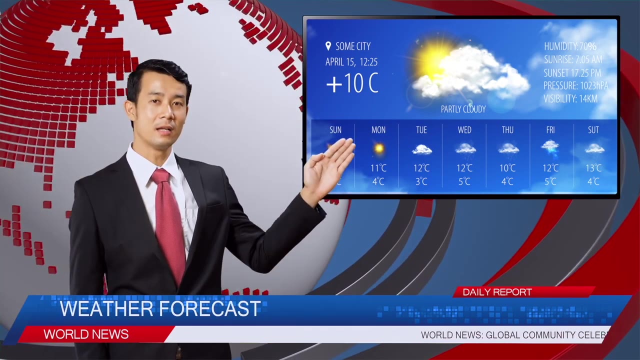 When was the last time you looked outside to see what the weather was like? Or maybe you checked your phone to see if it'd be a good day to get outside or go to the beach? Was it in the last 24 hours? The weather has such an impact on our daily lives that it's usually one of the first. 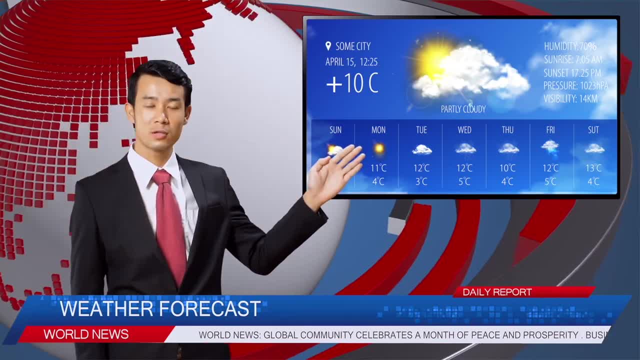 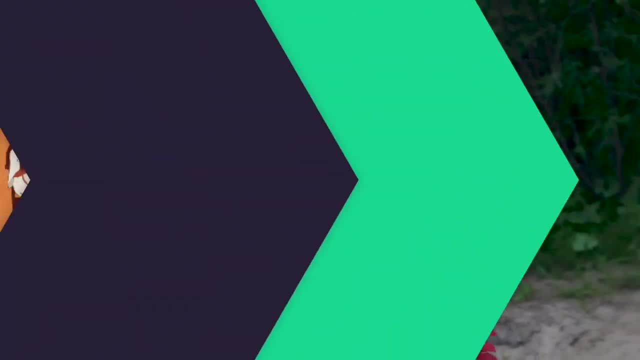 things we want to know each day. They even put it on the local morning news. It's one of the few things we share with our distant ancestors, from thousands of years ago In fact. the weather was often the topic of lots of early stories and legends.